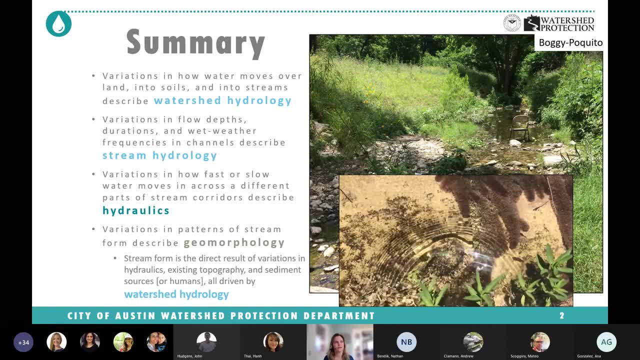 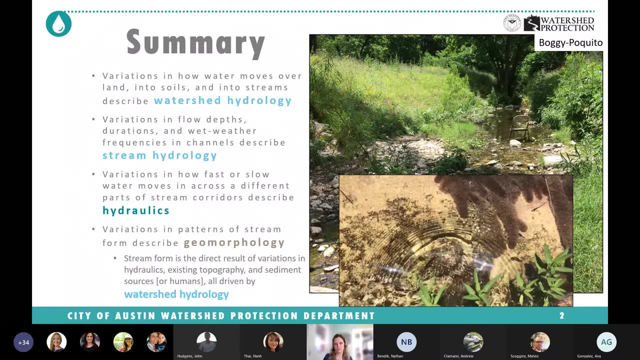 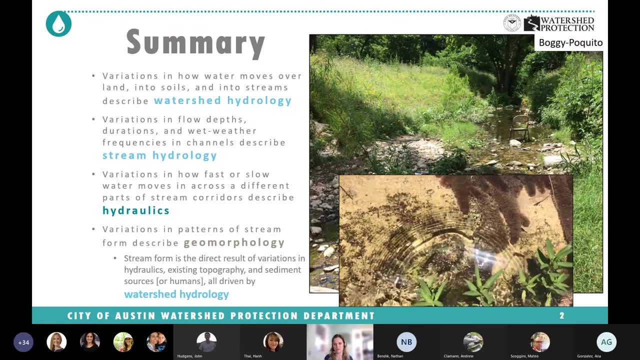 walk and talk through a stream or we've sat on a stream bank and kind of waved our arms a little. The takeaways are that watershed hydrology is just about how water is moving over land into the soil and into our streams and how that varies. Stream hydrology is about how 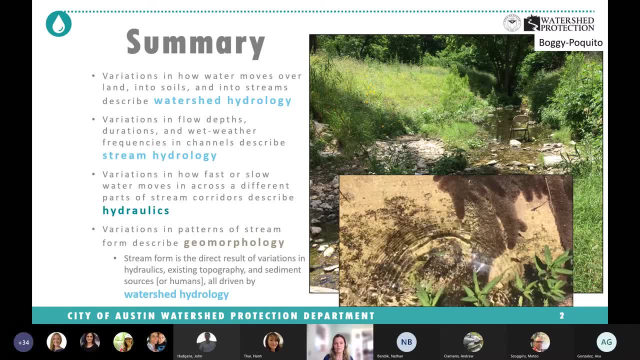 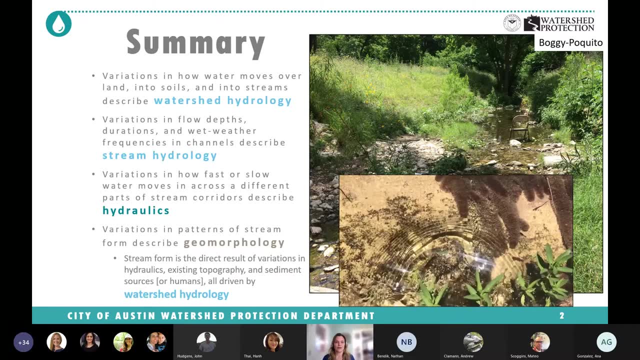 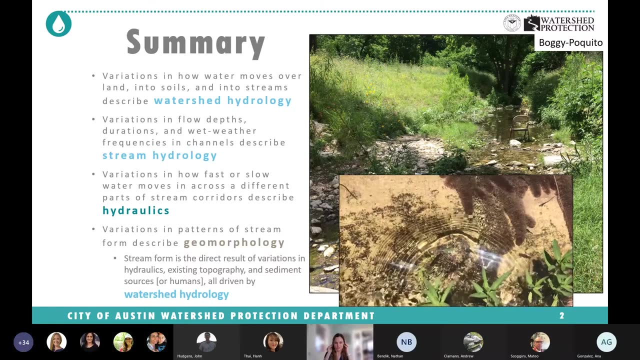 water is going varies in flow depth, how long, when are we getting those wet weather frequencies and how the water is being flowing through the river. And finally, hydrology is how fast or slow water moves across different parts of the stream corridor. And then, my favorite part, are the 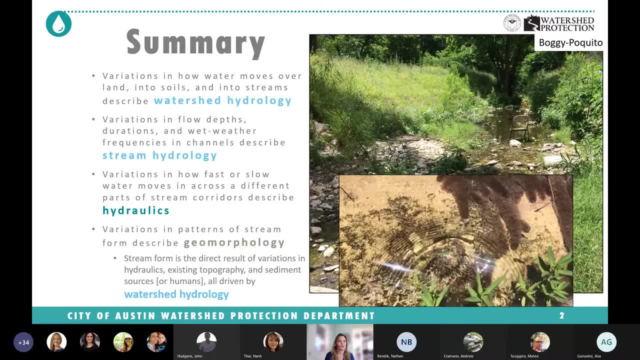 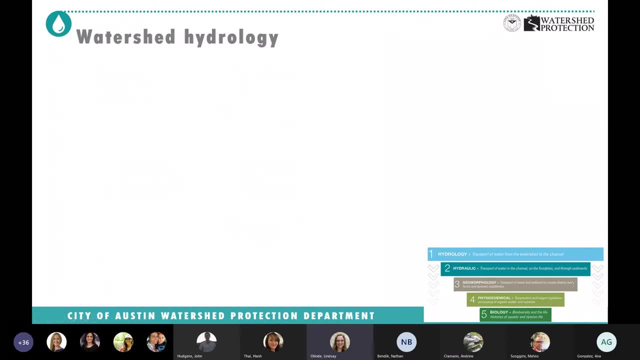 variations and patterns of stream form, And that's geomorphology, which is just a fancy way of saying what are our streams looking like. And I wanted to start off this whole talk with this idea of what a watershed is. Someone in watershed asked me the other day, like: at what point do we have a watershed? what size makes a water? 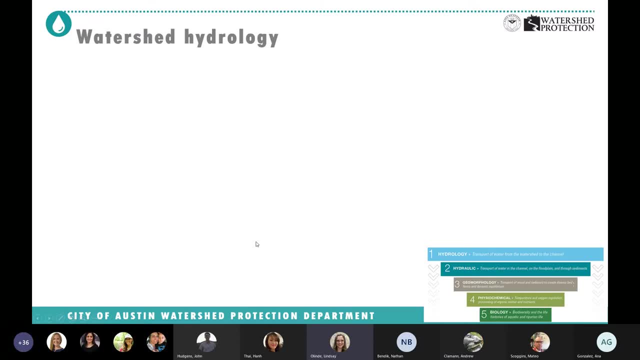 perfect, So I could stop here and I'll come back next week with an answer, if you think this is the right word for it. Okay, thanks, so much makes a watershed, And I think that's a really important um idea, because we have you know. 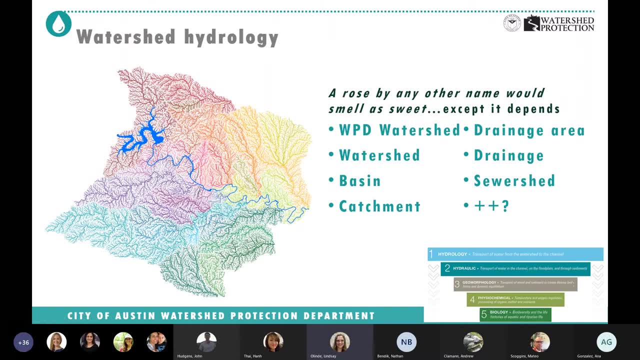 the capital WPD watersheds which are our kind of our boundaries, We can refer to: oh, we've got Decker Lake watershed, um, uh, Gilliland, but a watershed can be as small as a, you know the. 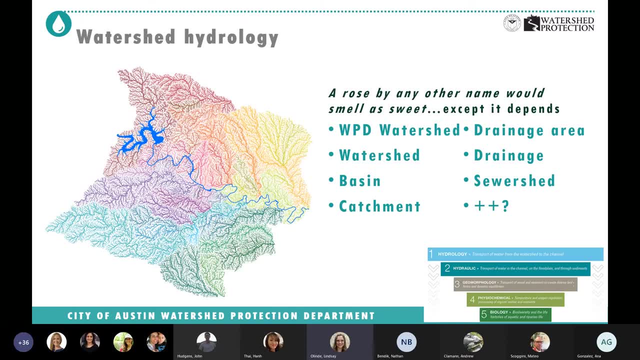 roof going: uh, runoff off your roof or as big as Onion Creek. So it really depends on scale And I just think it's a helpful thing for us to be mindful of when we're talking to community or ourselves. everybody has a different um kind of word that they like to use for watershed. 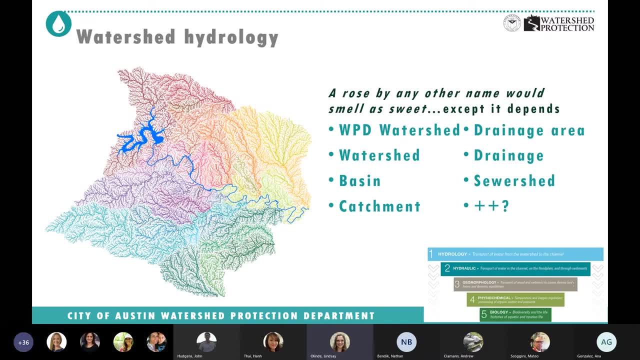 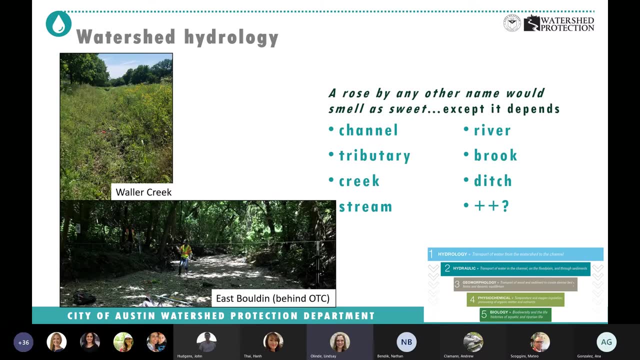 watershed, basement, catchment, drainage area, sewer shed. So I just wanted to lay that out there. and then similar for channel. you know, I grew up in the bayous of Louisiana So I had the Mississippi river and things called bayous, And then I worked East coast and West coast and I was always working. 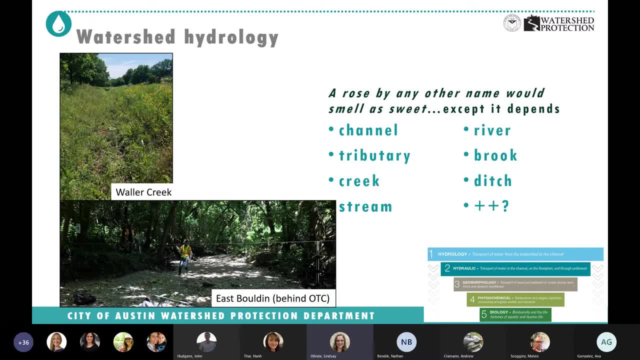 in um, streams, Um, and then I moved to Texas and now all of a sudden I use this word Creek. So I think that different people have different um images of what a Creek is versus a stream or a river or a ditch Um, and so I think that's another good thing for us to be mindful of. 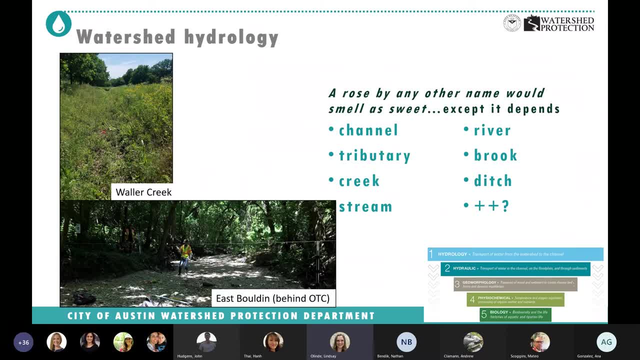 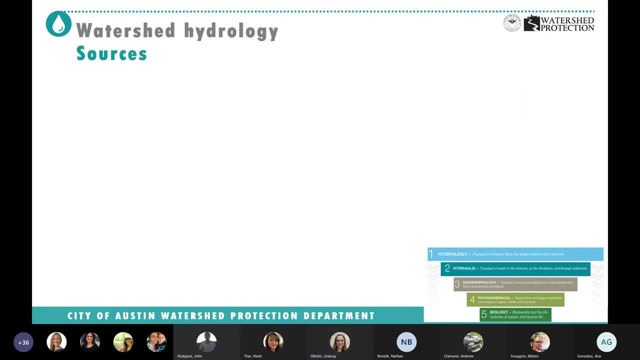 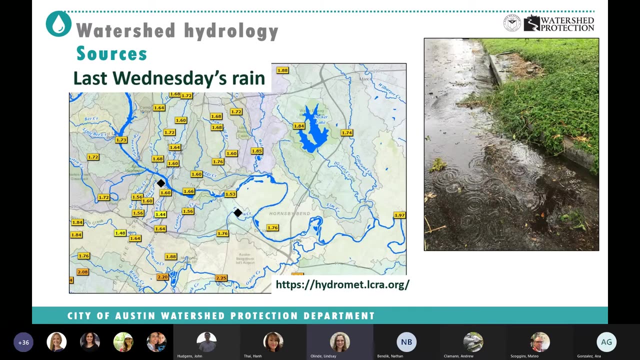 even when we're talking amongst ourselves or with the community. got Waller Creek, headwaters of Waller Creek here and East Bolden right behind OTC in our watershed. in Austin Our main water source is rain, So we've got last week's Wednesday rain from HydraMet. I have OTC. 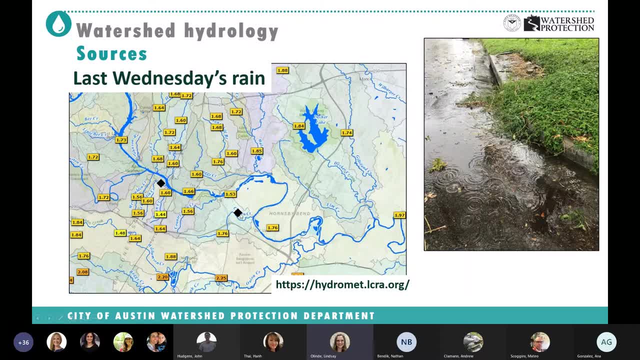 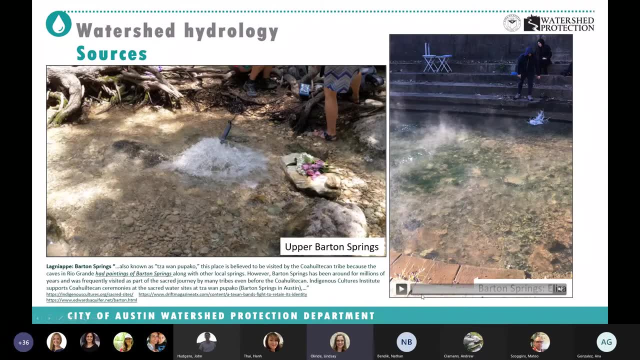 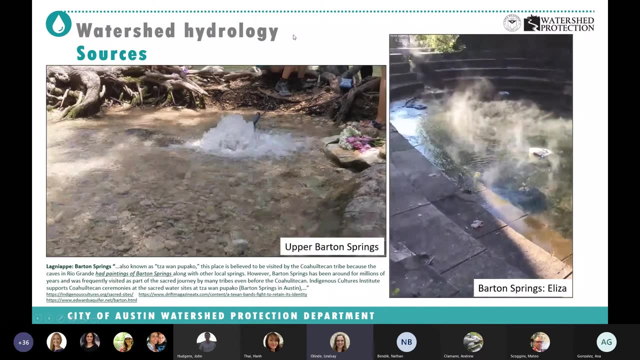 here and then Sherman over here. We've got about a little over an inch and a half of rain last Wednesday And we also have in across Austin. we have some springs, which we know well. here's some beautiful videos. Even in East Austin we have springs, shallow, alluvial springs. 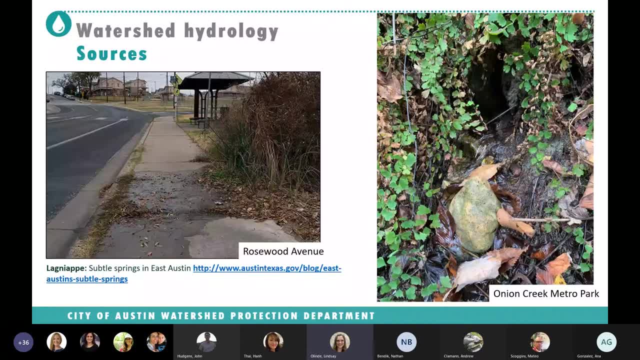 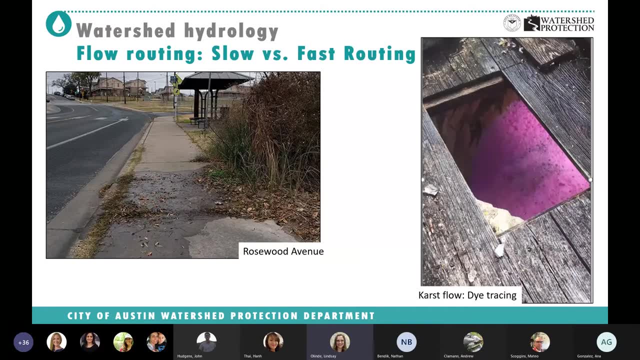 you know, which look different than where I may be used to. but you might think that they're a pipe, a little busted pipe. but all of those sources do eventually get to our Creeks, So that's another source. So watershed, hydrology, water falls, or, you know, comes out of a spring. 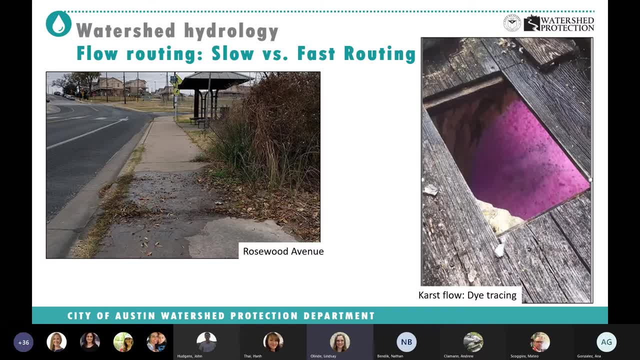 and they have fast routing and slow routing. So slow routing sometimes is through springs. This is an example of a dye trace, a well going through car systems and that routing can, I learned, be really fast like up to four miles a day. 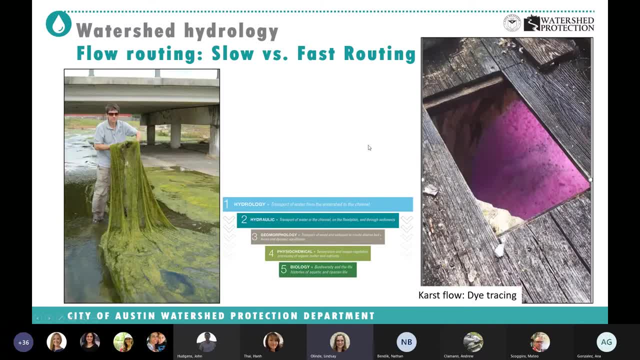 or a quarter mile per hour, at least a day of a mile a day. And then we have- it's important to know where everything that the water is flowing through on our watershed and what's picked up gets eventually into our stream. So here we have this. 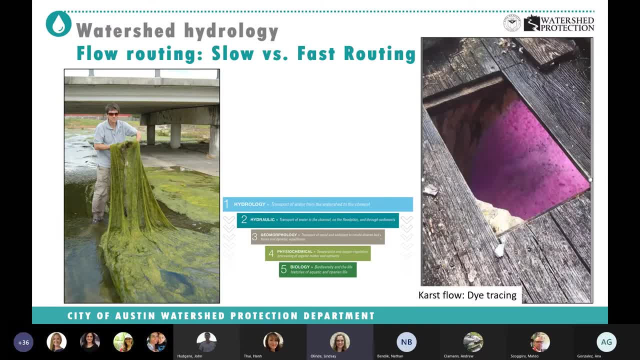 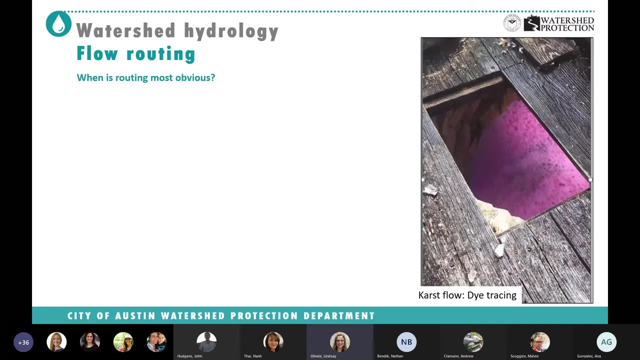 famous picture of Starin with some really well-fed nutrient-rich algae. Similar you can see it with the Trashiner Creeks. you know that's being picked up and moved downstream And for me the flow routing is sometimes not super obvious because I'm not often walking around in wet. 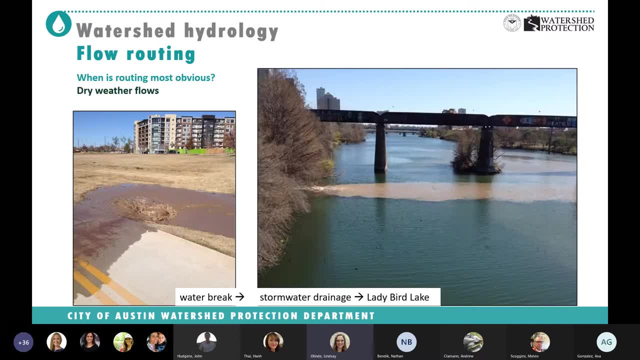 weather. Some of our crews definitely are, but the dry weather flows like. this is a picture from Spills where we had a water break and you could see that plume go all the way down to Lady Bird and we could easily follow it up. Sometimes slopes are so subtle even on streets. One thing I love: 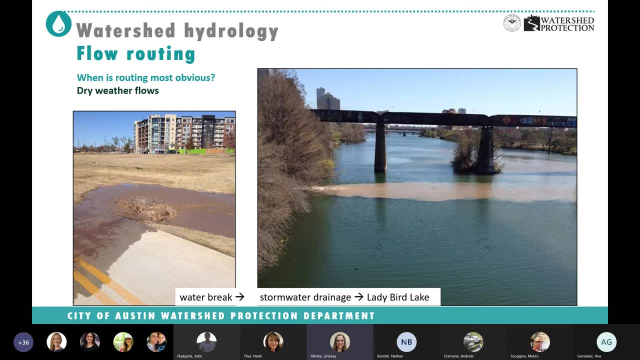 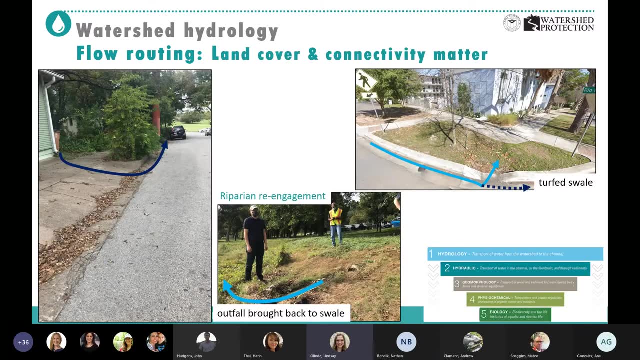 to do now is kind of walking around my neighborhood and guessing where would the water be going along the curbs and then wait for there actually to rain and see if I was right. So here we have kind of this typical roof to gutter to concrete all the way down and then right into 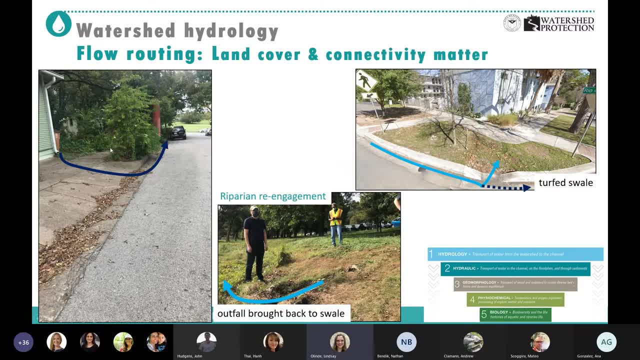 waller, This is about. you know, that's that kind of fast, really connected flow. And then we also have areas in town where we might have the. we can kind of disconnect that impervious cover. So we have flow and on our small frequent storms it can kind of flow into this little turf to swale that. 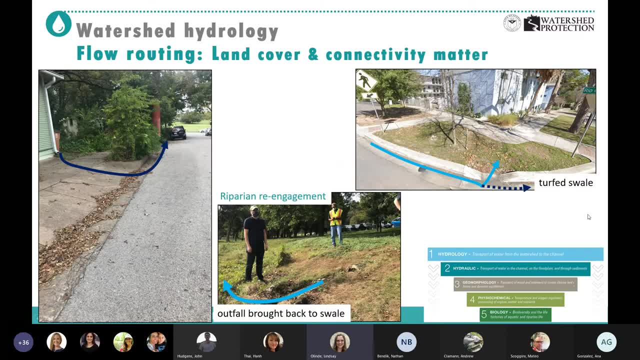 Tom made. And then when it's done, it's kind of like you know. it's kind of like you know it's too full, it'll bypass. And then similar in the Peace Park restoration. here's an example where we were able to pull back our outfall so that instead of dumping straight into Shoal Creek, 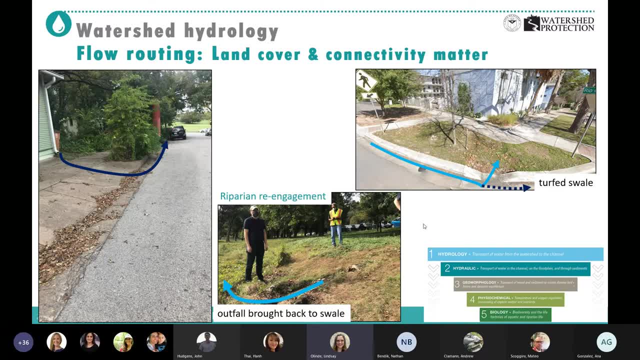 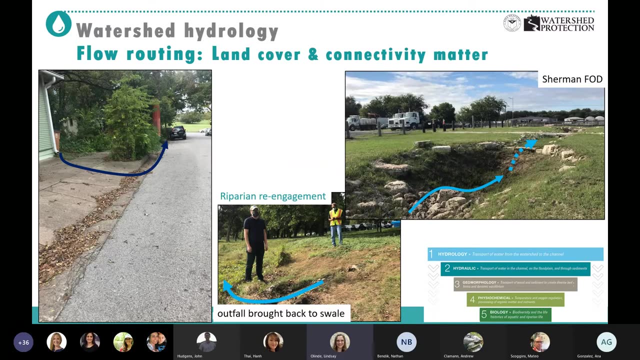 we were able to pull back, let them flow through the swale so that the water that was on the road isn't going straight to the creek. on these low or smaller, really frequent events, It doesn't even flow straight to the creek, It kind of slowly infiltrates over And then out in Sherman. 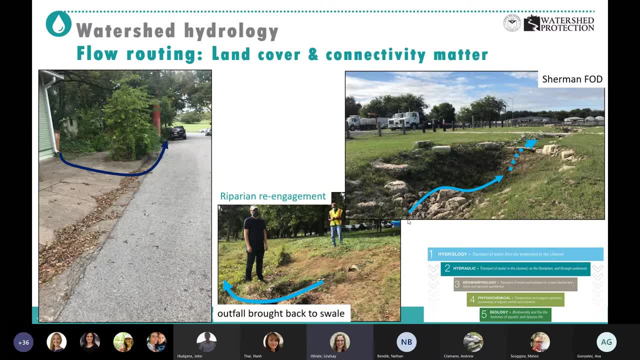 FOD looked like they had a lot of fun making these kind of depressions where the flow that they were intercepting from the site was flowing into these depressions And on these small frequent events it settles in right here And then, when it gets bigger, it'll go to this next depression. 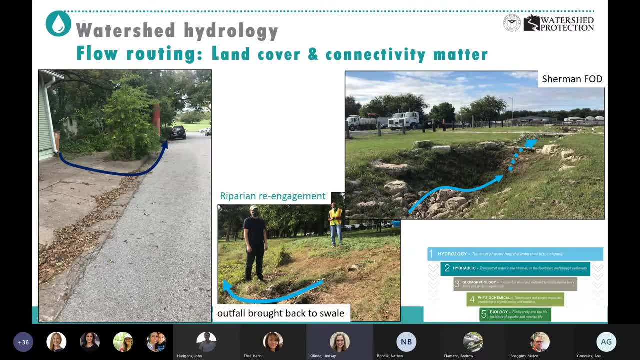 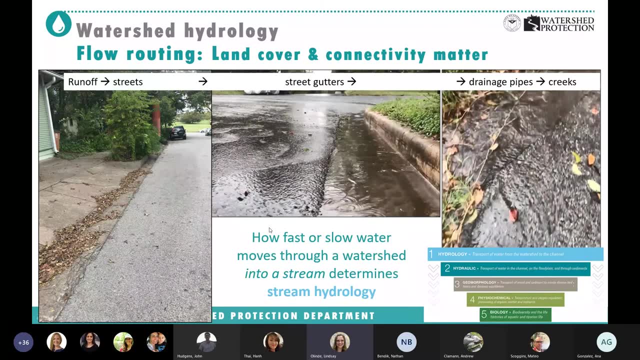 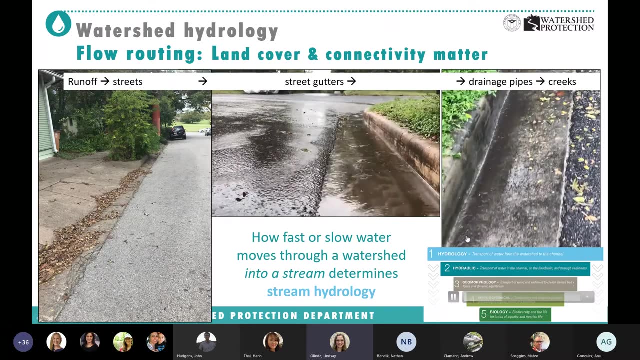 And then there's even a third. So that's another way where we can. these are obviously engineered, but you can get this idea that connectivity matters, So we have our street gutters. I was following some of the flows for our for this talk on Wednesday and I just started following them. 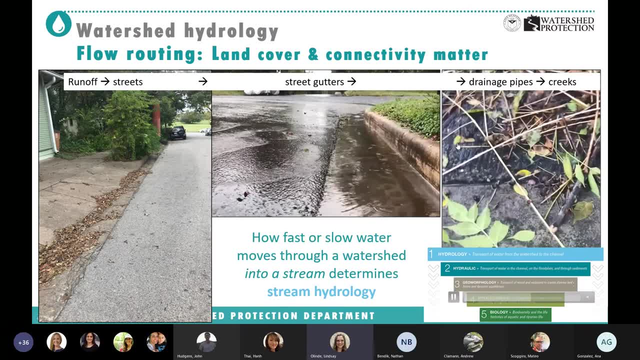 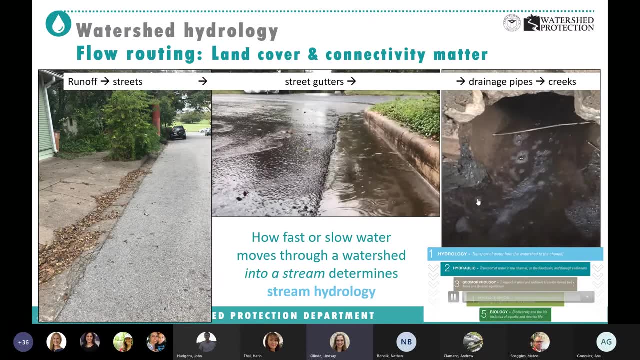 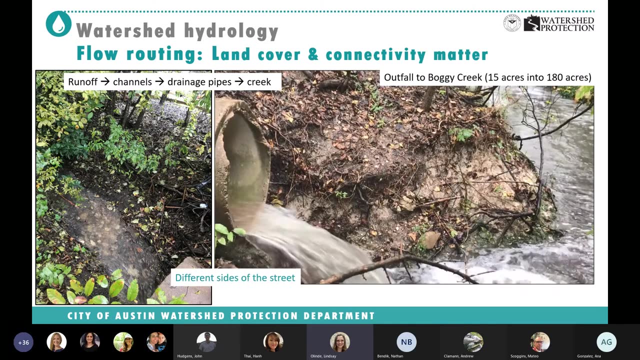 down watching it go into the curb And then, once it's in the curb, it's kind of, you know, pretty much going in general to our creek. So we're now we're getting into the stream hydrology piece And that's important because stream hydrology, this is the same. 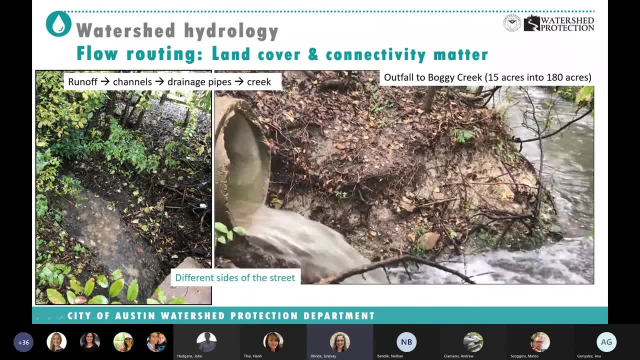 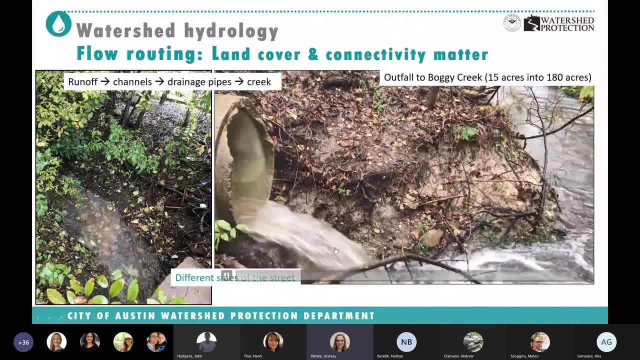 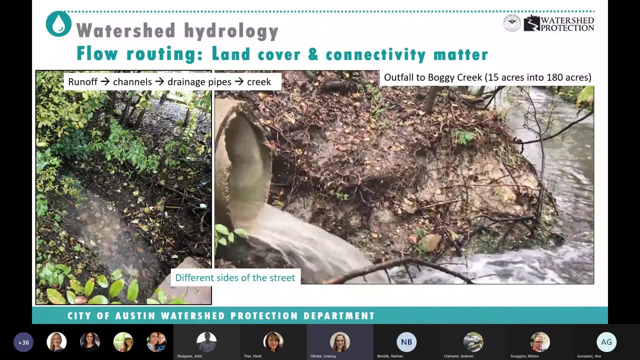 trib different sides of the street where our stream hydrology. really it matters how fast the water is getting here, how frequent water is getting here. Before we had impervious cover, you know we'd have. we would have a storm, a small storm really frequently, and maybe not all. 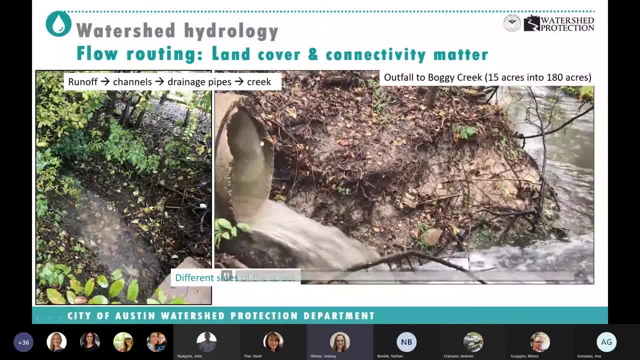 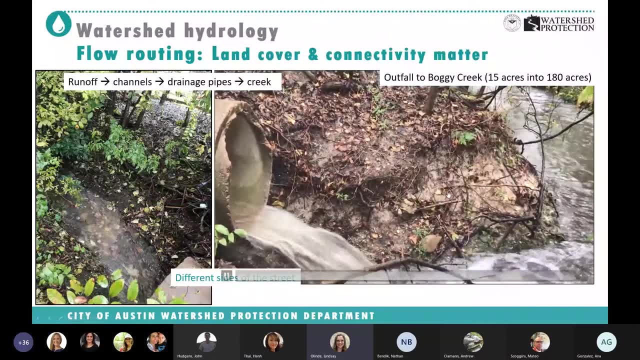 of that water would go straight to it. This was in the beginning of the Wednesday flow And it was not. there wasn't a lot of rain, but on the creek side it I would have guessed that there had been a lot of rain, So you kind of get those pulses. Similar place: we have an enclosed culvert where 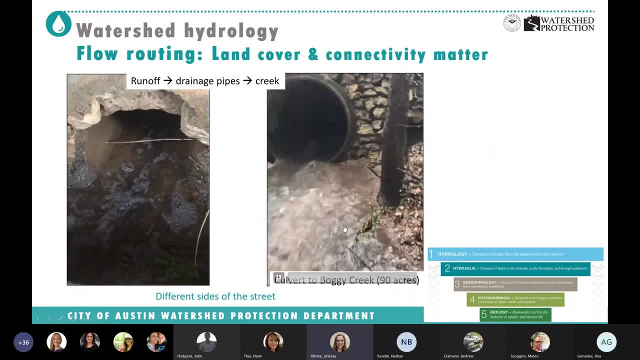 the stream is, So we have a lot of rain. but on the creek side we have a lot of rain, So we have a completely enclosed, pretty much 90 acre drainage And we have a lot of flow. And this was just the. 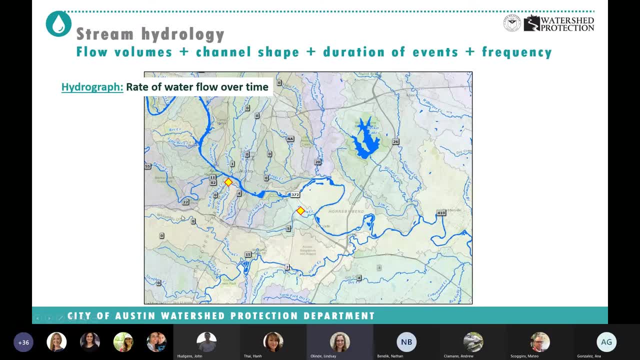 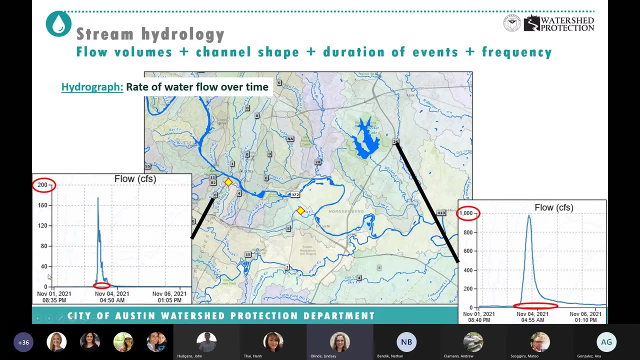 beginning of that storm on Wednesday. The hydrograph is just where we are, depending on where we are, this rate of water flow over time. So we've got our OTC and Sherman for reference. This really depends on what a hydrograph is kind of, what the stream is feeling during an event. This was a 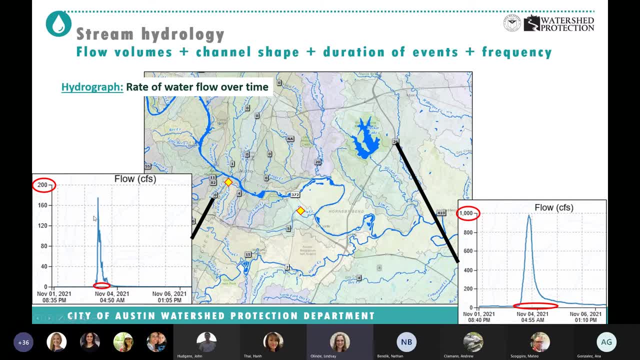 Wednesday. So kind of close to OTC We have a lot of rain but on the creek side we have a lot of pulse And then it went down. closer to on Gilliland We had an even larger pulse and then went down. So for the hydrograph with the stream is experiencing depends on the how high the water 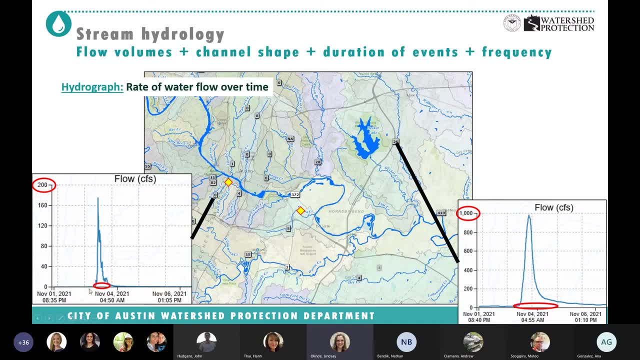 is getting So that flow depth and also like how long that lasts. So when we're getting these small frequent events, sometimes we get a pulse every single time if it's really highly connected And this is just a plug for we can get water alerts to your tech on your phone with text. 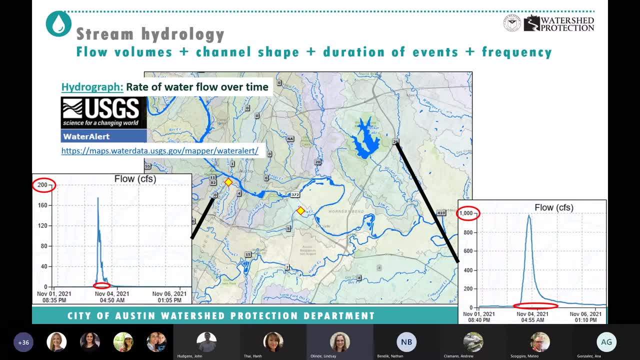 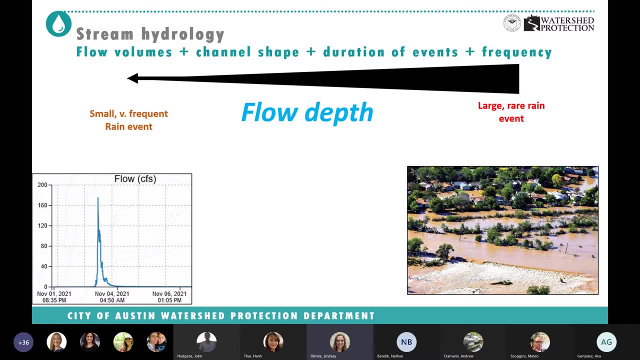 messages And I think those are really fun. I'm just trying to get an idea of what's going on around town or project sites And frequency is really important in streams. So part of the stream hydrology again is how we have an event from last Wednesday. We know intuitively that it wasn't as 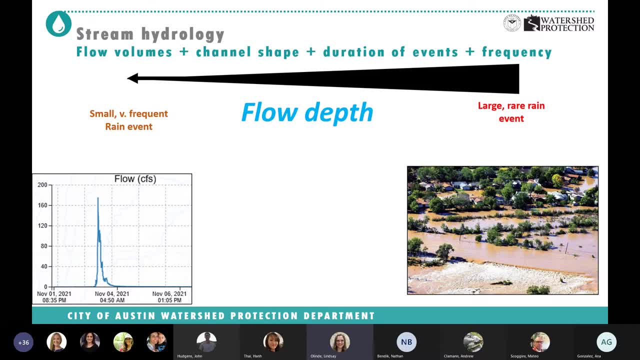 large as that kind of more rare Halloween flood back in 2015.. So how often are we getting high flows? How often are we getting these low flows? That's all about frequency And we'll depend on stream hydrology, which depends on watershed hydrology. I love this. 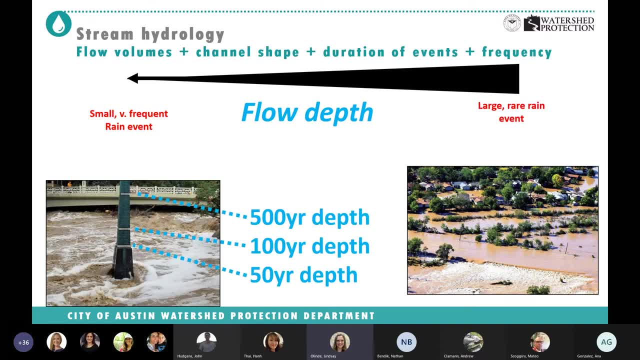 visual. This is from Boulder Creek. after one of the big Boulder floods in Colorado, They installed a art, piece of art that kind of helped the community visualize frequency and flow depth. So this was 50 years. This is a sculpture where it shows the 50 years, the 100 years and the 500 years, So that 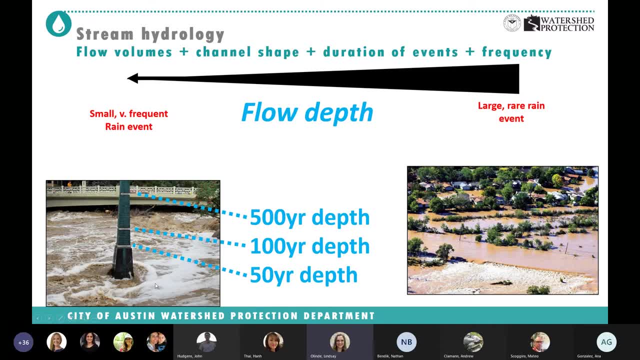 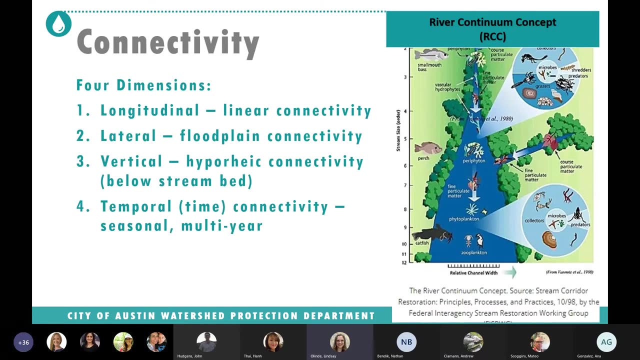 folks can kind of walk the green belt Or while it's having a storm and kind of get a gauge of oh yeah, this was a lower event compared to what they had before. So I think that was a nice way of thinking about flow depth and frequency. Now I'm going to turn it over to 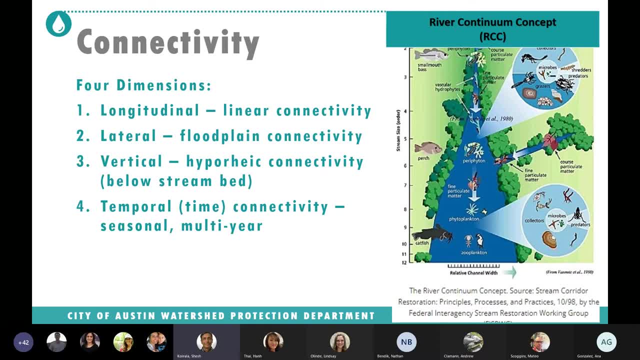 Shash. Connectivity refers to the flow exchange and pathways that move organisms, energy and matter throughout the watershed system. These interactions create complex but interdependent processes that vary over time. To understand the connectivity concept, it can be described in four. 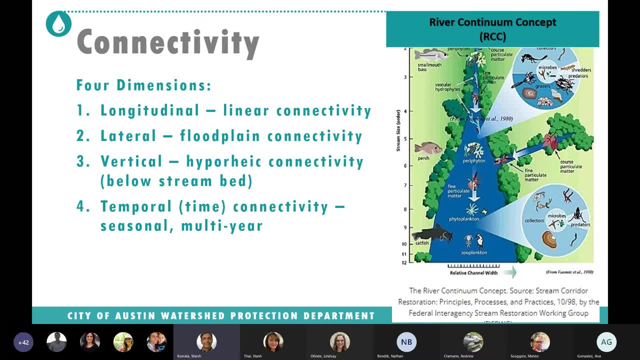 dimensions: Longitudinal dimensions, which is the linear connectivity, that is, the connection from headwater to the mouth of the river, And the lateral connectivity is basically the floodplain connectivity with the main stream, which I will explain in the next slide, And vertical connectivity. 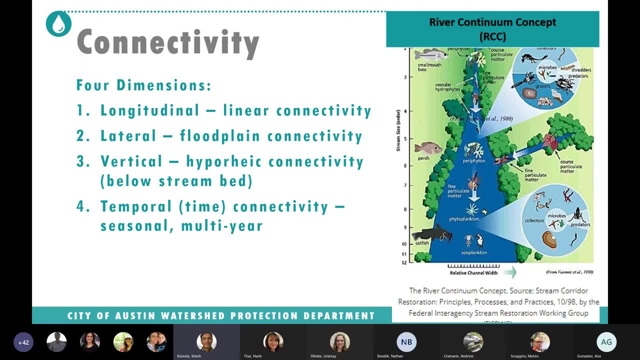 we call it as hyperlink connectivity primarily refers to below the stream bed and groundwater connectivity with main stream And, of course, the last but not the least, is the lateral- and I mean temporal- connectivity, which is the connectivity over time, with many scales like seasonal, multi-year, let's say two-year, five-year, hundred-year, that kind of things. 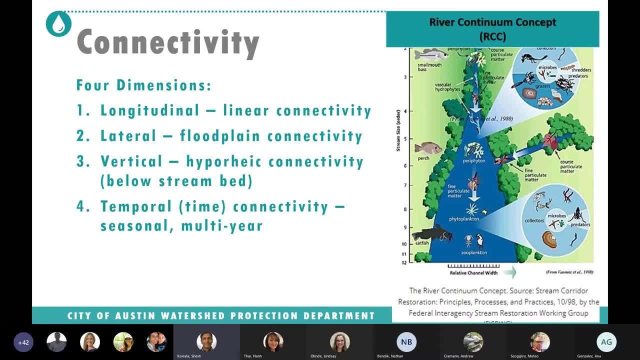 that connectivity. This connectivity concept is based on river continuum concept, which is a model for classifying and describing flowing water, And this is a concept of dynamic equilibrium in which stream functions are in actually balanced between physical parameters such as width, depth, velocity, sediment load and also taking into account some biological 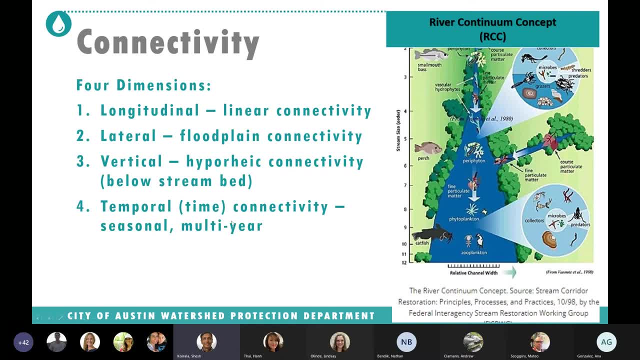 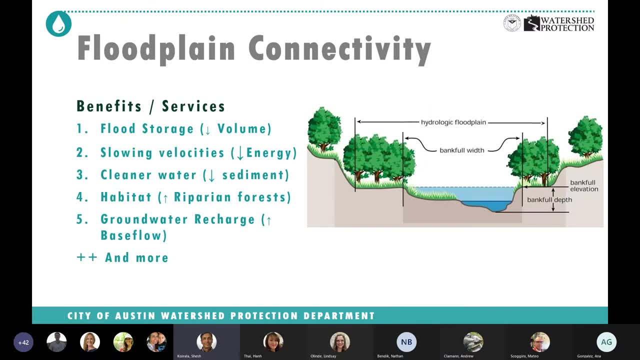 factors. This is a holistic concept and was developed in early 1980s. I'd like to go a little more detail on lateral connectivity, which is basically the stream floodplain connectivity, as I mentioned in the previous slide. Lateral connectivity allows the stream access to its floodplain during high 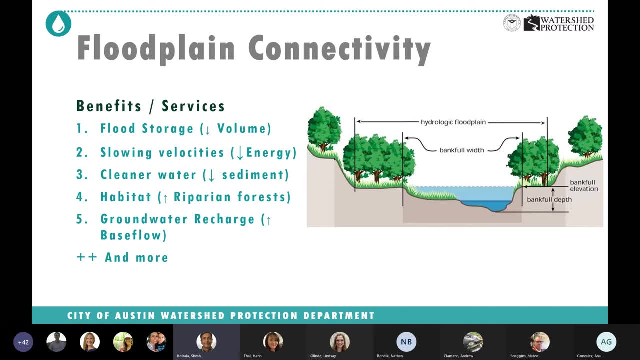 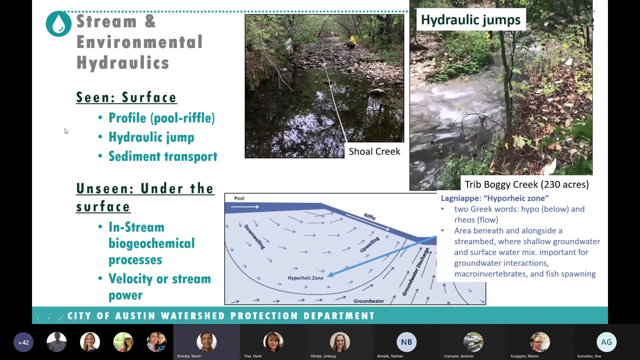 water events. This access is critical for the healthy ecosystem function by exchanging nutrients and other organic matter to and from the stream. There are many benefits of this connectivity, such as flood storage, cleaning of water, groundwater recharge, increasing riparian forest, which is very important for the habitat, and much more actually. Let's go a little deep into. 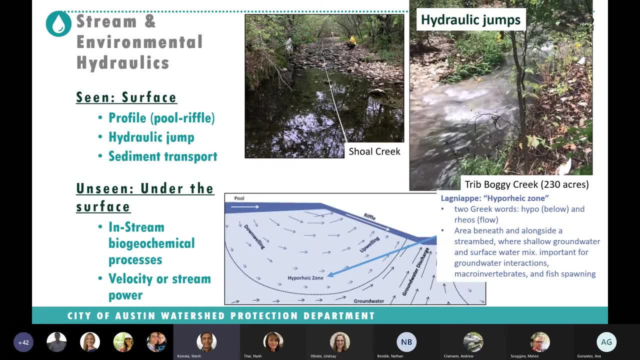 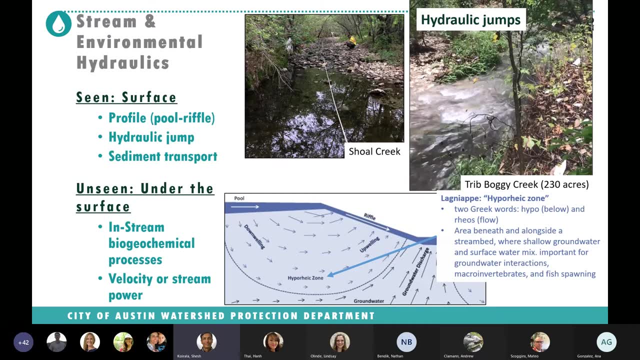 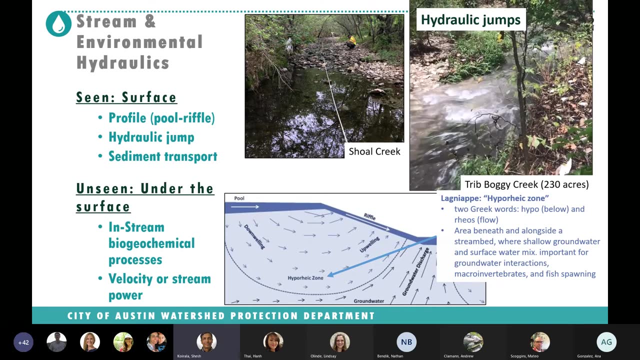 stream, environmental hydraulics, When we go to a possibility- and I'm talking in the context of urban- the stream and see what, what? what we can see is basically the pool and refill and we see the hydraulic zone and if the creek is muddy, we see the sediment, pool, refill, occurrences, occurrences. 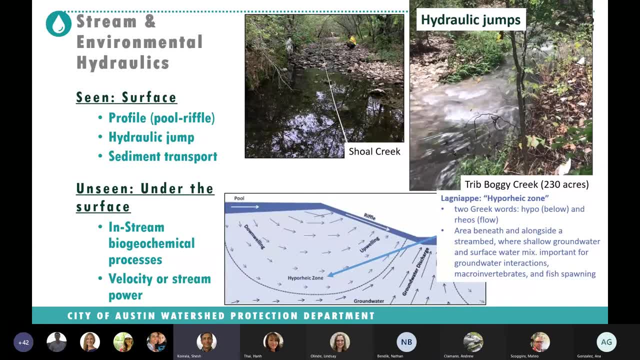 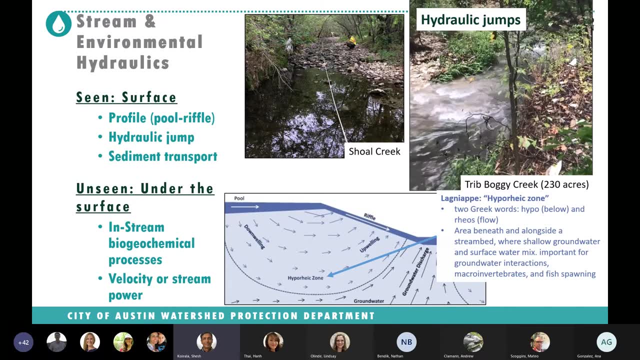 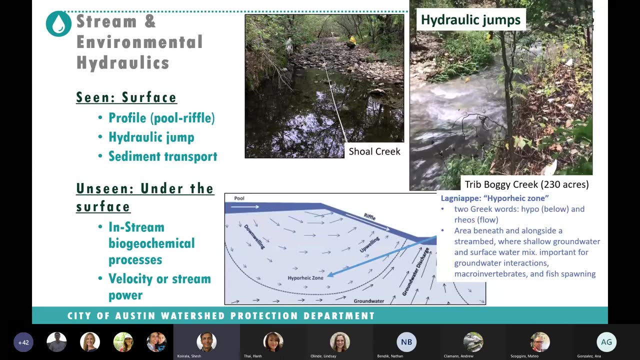 like depend on the geometry of the channel, basically the slope of the channel and the velocity of the flow. in any natural stream there is a sequence of pool and refill which is really important for the stream's overall health. when the stream water flows from a steep slope to a very 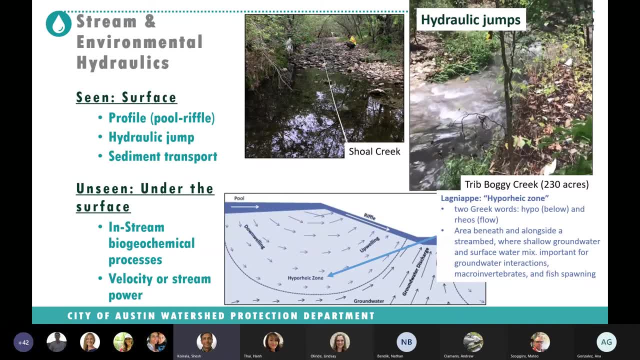 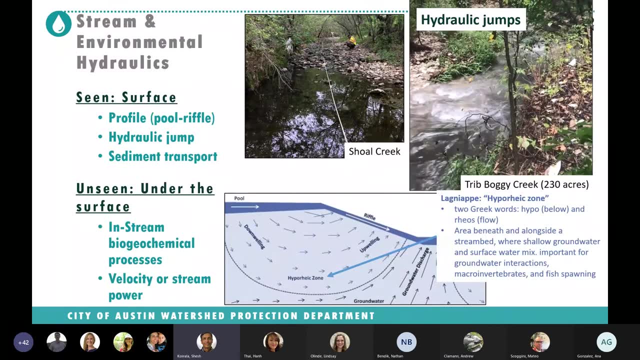 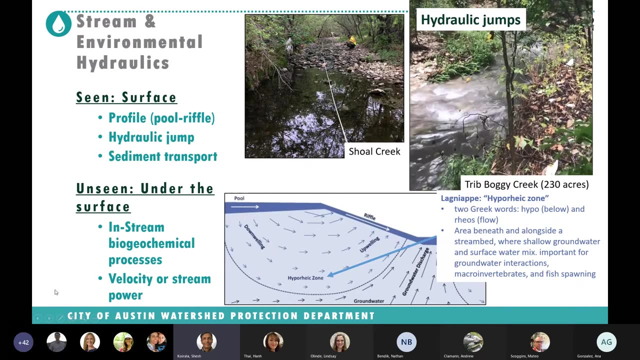 mild slope. at the bottom of the steep slope there is a swirling of water and it's called hydraulic jump pool refill and hydraulic zone type of phenomena are important for maintaining the dissolved oxygen level in the stream. there are a lot of things and processes happening under the surface which, of course, we cannot see. 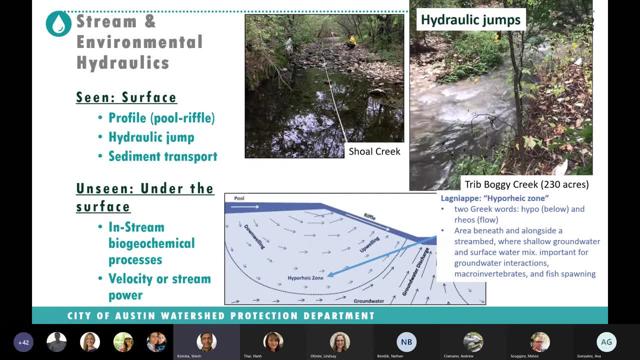 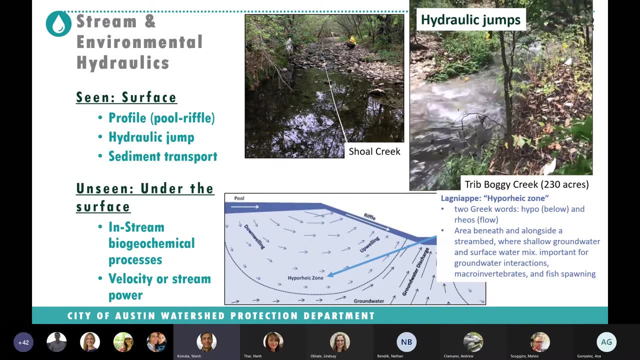 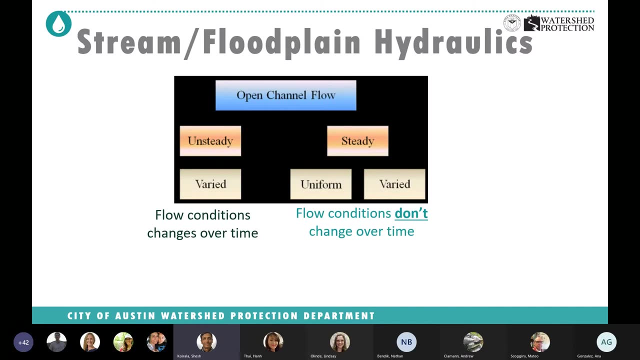 these are in-stream biogeochemical processes. we can guess, but we don't know what. what's the velocity of the stream and what's the stream power? these are very important parameters to estimate the erosion potential of the stream. let's let's go more detail on stream and floodplain hydraulics. 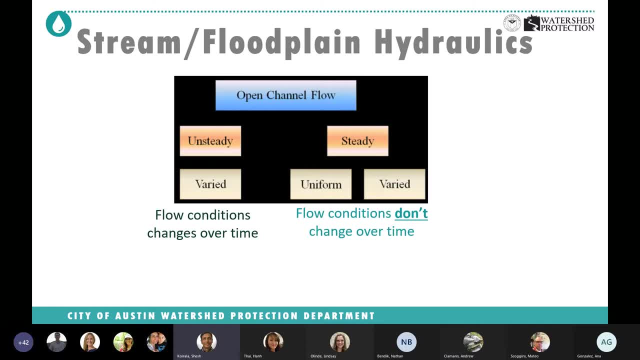 we call the stream flow is open channel flow. this flow is divided into steady and unsteady flow. if the flow- it it certainly section- is constant over time, it is called a steady flow. otherwise it's on a steady flow. in the steady flow, if the velocity is not changing at different sections of the stream, it is called 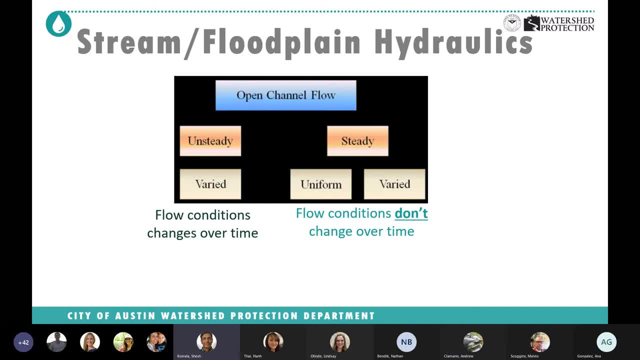 the uniform flow. otherwise this is varied flow in in in both of these categories. depending on how it is changing, they are divided into gradually varied and rapidly varied flow. roughly speaking, if we consider a base flow of a stream, it is steady, uniform flow in a strong event when there is first increase in the flow and then 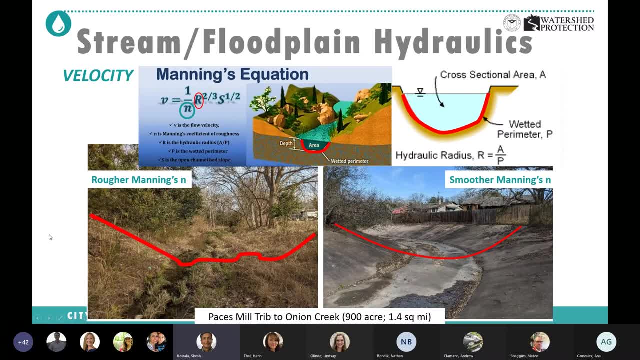 decrease. it is primarily the unsteady flow. the main objective of stream and floodplain hydraulics is to find out the velocity of the flow in the stream and floodplain. for this manning's equation on the picture here on the left is used. this equation was developed in actually, 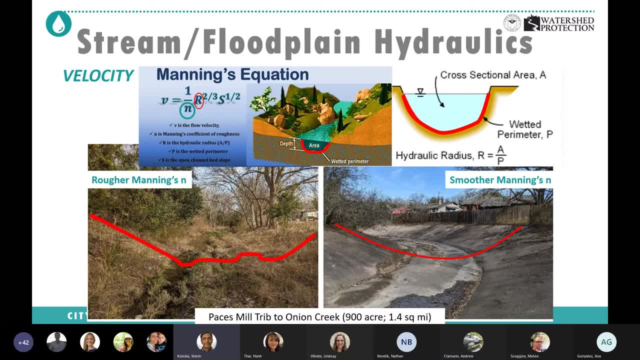 1889, about 130 plus years ago, but we we are still using this for modeling. as you see here, the velocity depends on geometry of the channel, slope of the channel and basically the roughness of the channel. if the roughness is high, just like in the lower left picture, like with the grass lining, 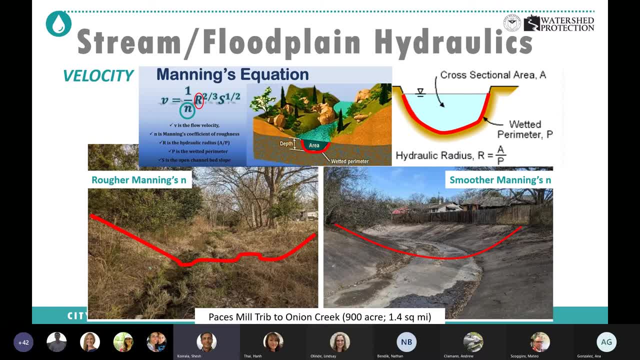 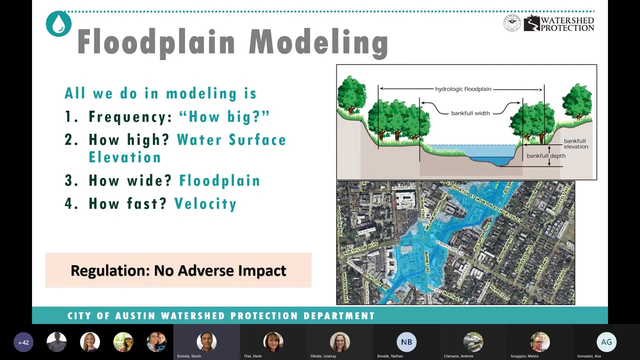 velocity decreases, and if the roughness is low, like in the concrete channel, engineered channel, velocity increases. uh, but this is this looks obvious to to all of us. this equation used to quantify this velocity. all we do in plot and modeling is to find out what is the frequency of the storm which basically comes. 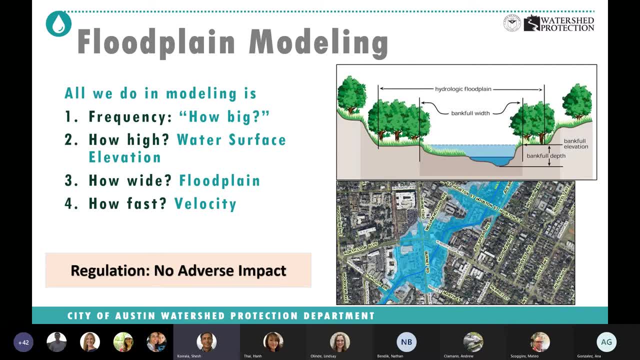 from the storm event for rainfall and how high water goes in the stream in the floodplain and how wide it is spaced in the floodplain and how fast it moves these poor things. basically, as i mentioned in in the, i think, in the previous slides, how important floodplain is to keep the 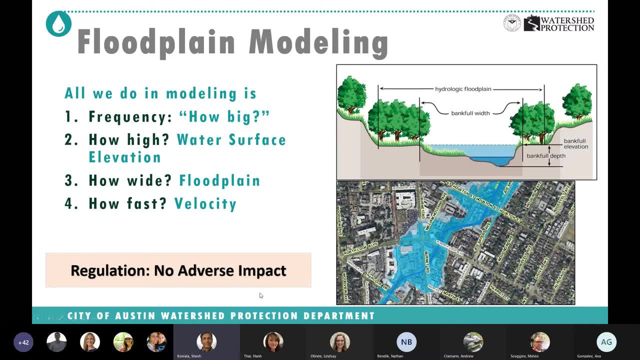 stream and watershed healthy. through our regulations, such as drainage and environmental criteria, manuals and land development course, we make sure that there is no rise in water surface elevation, there is no increase in floodplain width and there is no increase in velocity of flow that actually that may cause it partially to the opposite. 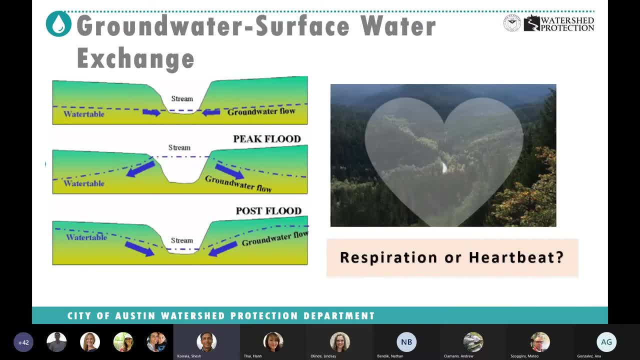 downstream and side neighbors. This groundwater-surface water exchange is the vertical connectivity that I explained in my first slide. There is a continuous exchange of surface water and groundwater from end to the stream. Along with the water, there is an exchange of nutrients as well. The exchange rate and 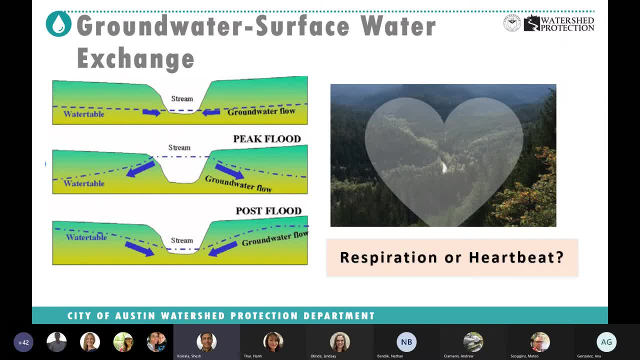 the direction of the exchange give and take follows the same principle of energy flow: from high energy to low energy. In hydraulic terms it is called the hydraulic grid line. In the stream it is the top of the water surface and in the groundwater it is called water table. Water table is. 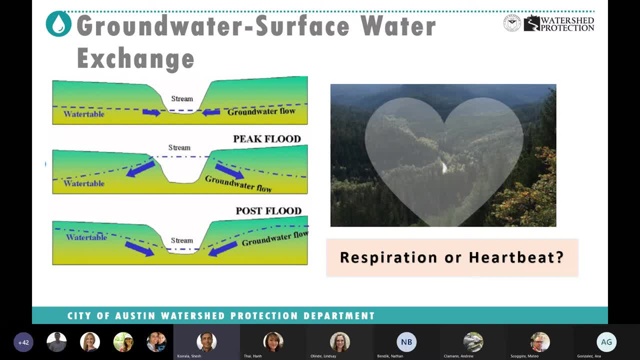 basically the boundary of saturated and unsaturated ground During peak flow time after the storm event. as you see from the second figure from the left, the flow of water is un-saturated, The flow is directed to the stream and ultimately maintains the base flow. 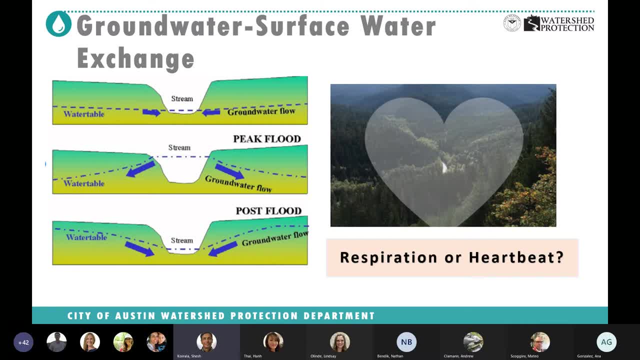 condition in the stream. Then the cycle repeats with this exchange as the stream flow increases after rain events. Don't you see? this is a pump in and pump out, just like our heart. I think it is This inhale-exhale type of phenomena is. 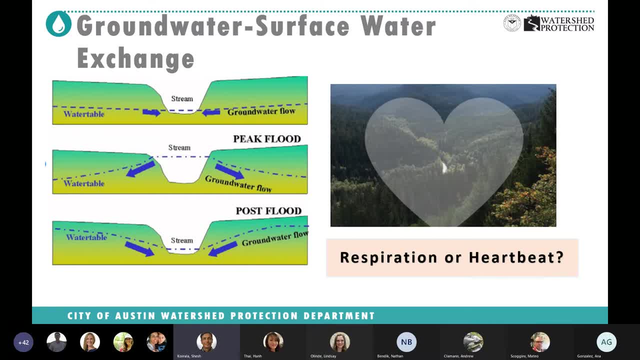 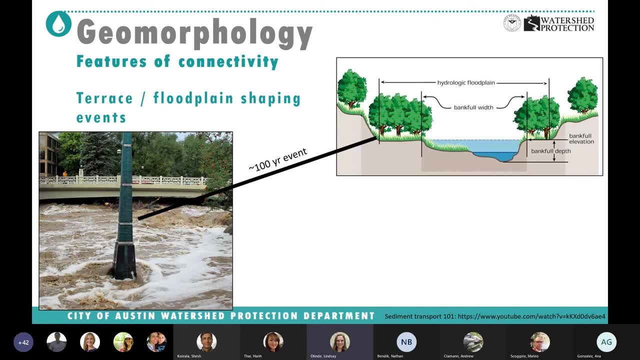 important. It is important for stream connectivity and overall stream health. Now I give back to Lenshi. I love the analogy of the inhale-exhale on that Carrying through with this stream or river corridor concept where we have this is a cross-section of a creek that Shash was showing. 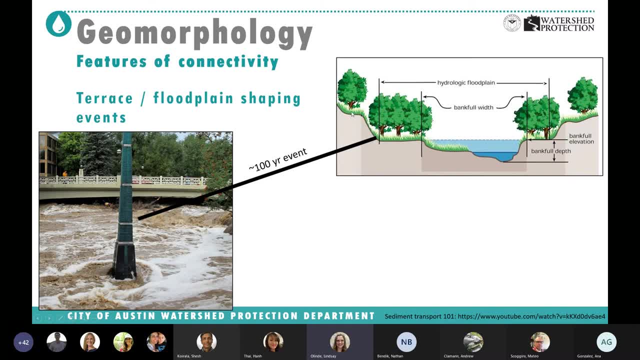 we do a lot of modeling and a lot of regulations and thinking about the 100-year event And those large water howitzer divisions are really big or more than a 100-year event also. That's really what can shape our kind of larger scale valleys or our terraces. The smaller events are actually. 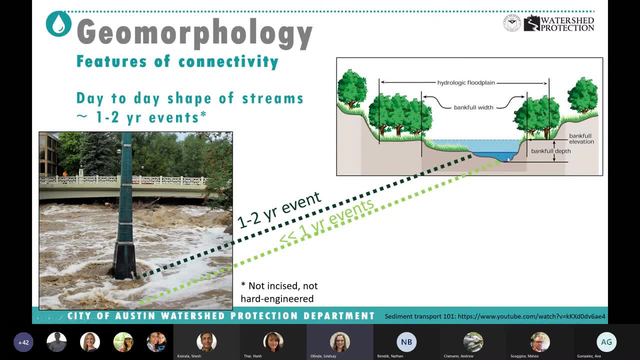 what shape the primary flow path that we see during our less than 2-year flow. Some people call it bank-full, And it's these especially low events that are in the kind of the middle of θα faster part of the channel, that are really ecologically and geomorphically important. 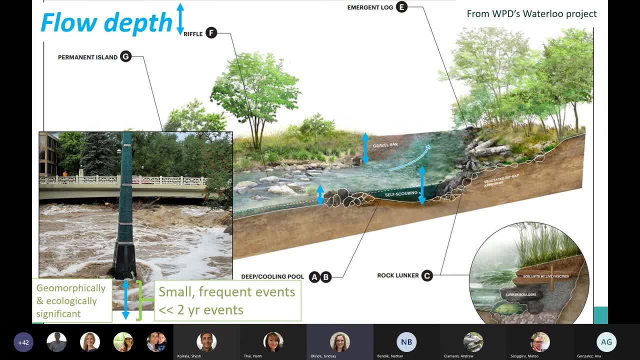 I have been really loving this image in terms of geomorphology and stream corridors that came out of Watershed's Waterloo project. It's a kind of 3D cross profile, cross sections that help look at breaking down different features that we might see in streams. So here's an example of a riffle. 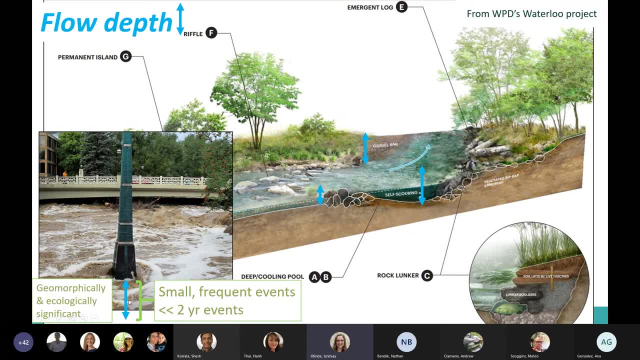 We have some scour pools And you can imagine that in these smaller events, as the flows are going up and the flows are going down frequently, we start to engage different features. So, for example, when we have our smaller frequent events, maybe we are having flows through the riffles. 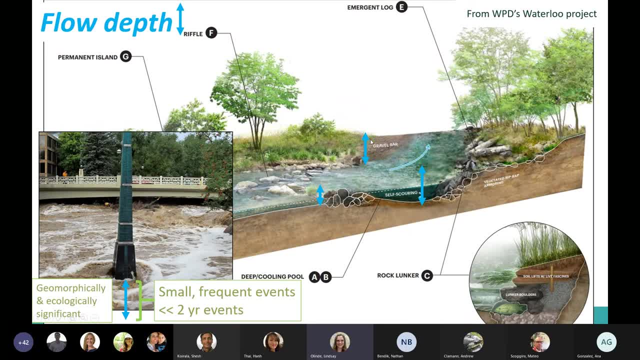 If we are starting to raise it even beyond, then we might be starting to get flows covering the gravel bars that we're seeing And, as we have higher depths, we might be starting to get into these kind of low bank height or a little bit of floodplain interactions. And I just shout. 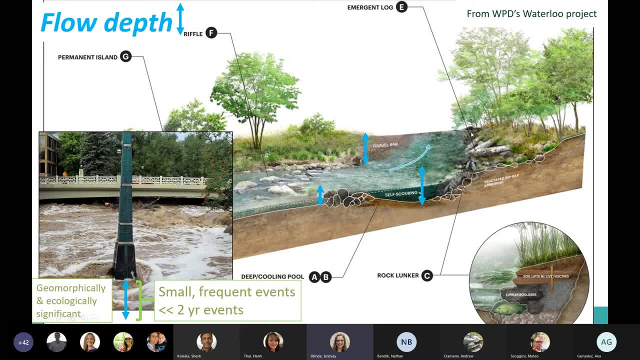 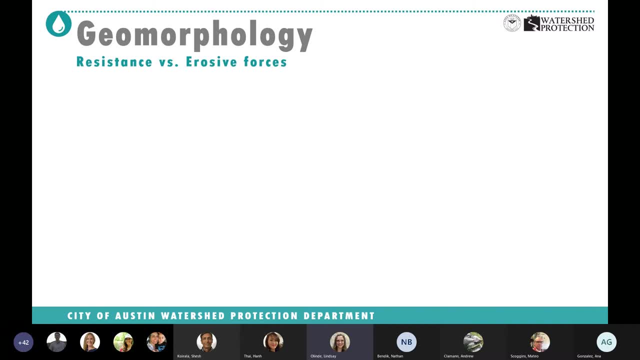 out to the Waterloo team. I have been really enjoying that Going from stream hydrology into geomorphology. Geomorphology, and how the stream looks to us, is really this trinity of sediment, Topography and flow or hydraulics, And for me I think a lot about when we go to a site, kind of 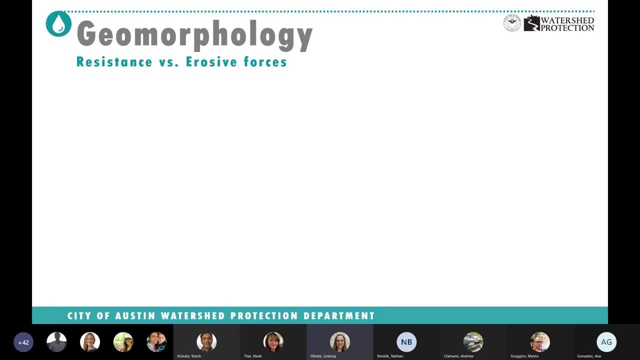 reading the creek, we can look at different indicators and we can generally see what is the balance between our resistant forces and our erosive forces in terms of if we're having- you know- I'm kind of focusing here on when we go to a site and we're having- some kind of 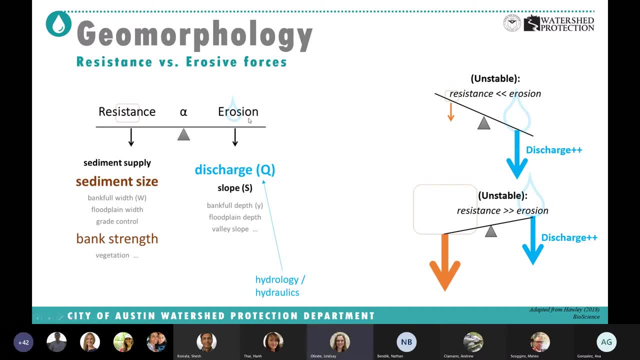 instability issues, Because that's often what we're trying to repair. Our erosive forces have to do with discharge, slope, that velocity driving that can pick up sediment And, depending on how the stream, beds and banks are, that's that resistance force, So we can have unstable conditions where we have. 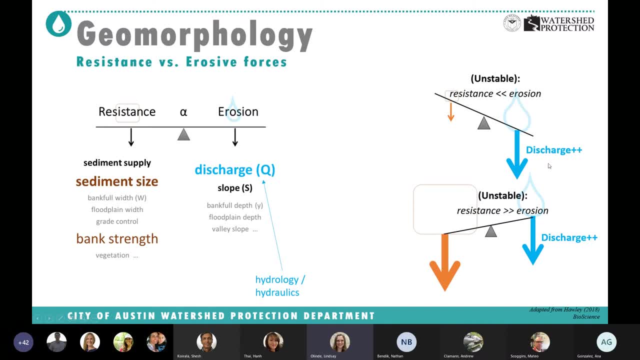 really high discharge now, whether it's from now we have a lot more impervious cover that's go that originally wasn't in our stream. So the stream, the natural stream beds that we have, can't resist that, And then we can also have areas that are 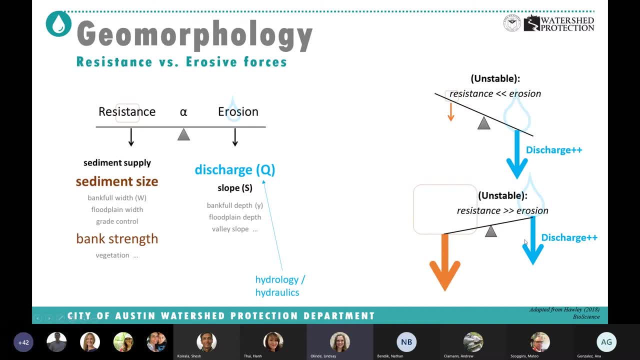 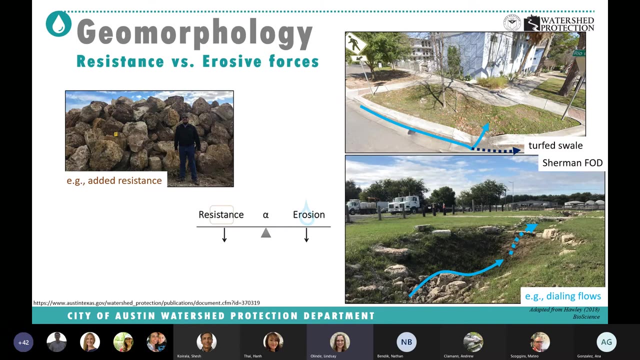 unstable, where we are having the same amount of discharge, but now we're having so much sediment that maybe came from upstream that that sediment is getting deposited and the discharge isn't able to keep carrying it. We are trying to create a lot of balances from resistance and erosion as part 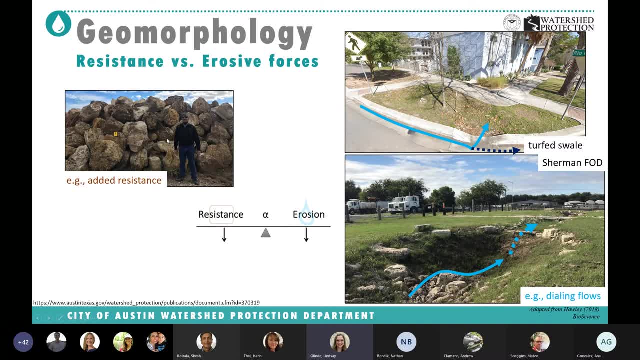 of our work. Sometimes we add resistance. This is a great picture of Eric Lauchs at Sherman with some mega 36 inch grip wrap that we might add to some places that we really don't want to have the stream bed change. And then we also have a ton of SCMs out there. We have detention ponds. detention pond. 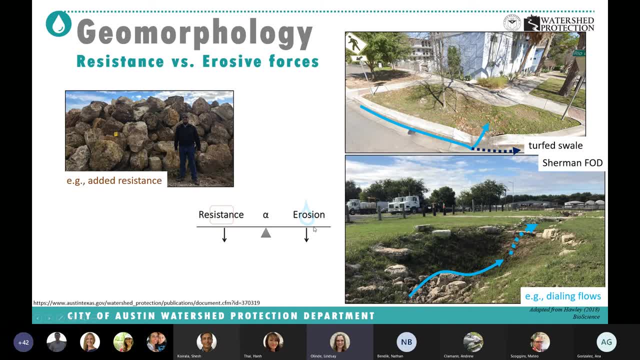 inspections are critical because we are expecting these ponds to hold back water. We have even smaller scale options where we have- this is an example that Tom did on the 18th- and grant and Rio Grande, where the flows on our small events are actually captured and kind of stay in this. 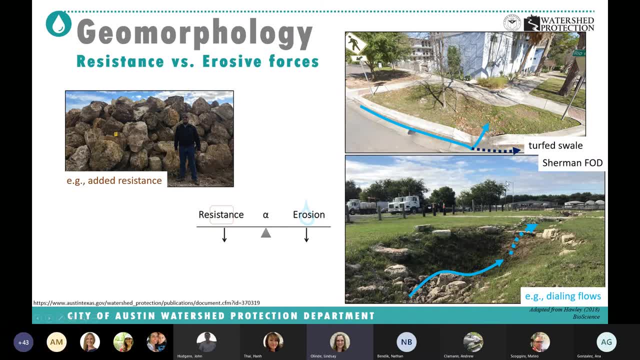 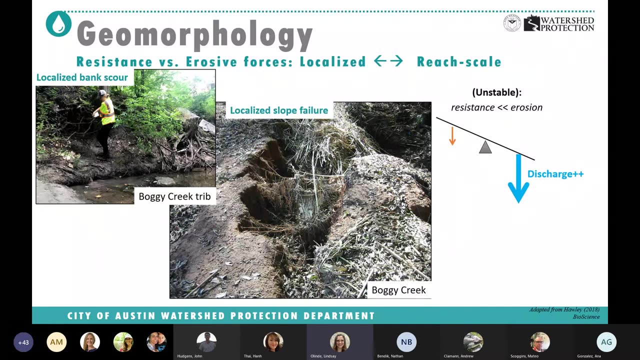 turf swale and on the bigger ones that keep, they are routed into the streams. We also have again the Sherman, where Sherman started flowing, catching some of that flow and not having it go into Carson Creek. This is some examples of localized issues that we have. This is here's. 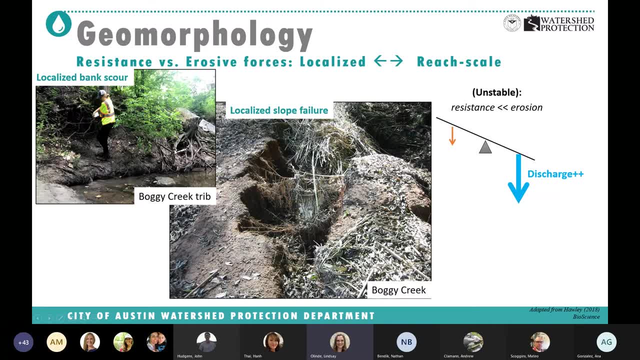 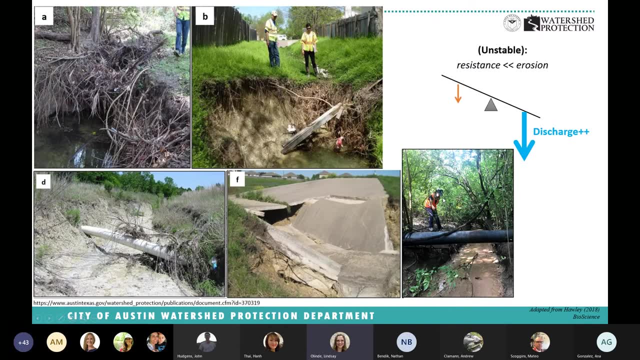 a picture of Ingrid and Boggy trip where we've got some scour going on some bank failures. This is looking down down watching bank failure of some sloughing off. Here are just our more examples kind of our, of our, some of our problems. We have incision when we have too much discharge and not 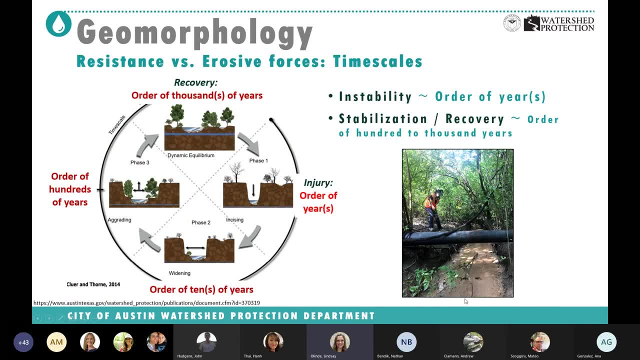 enough bank resistance, classic head cut. A lot of our responses are fairly acute. They happen fairly quickly And if we're going to let it kind of equally become stable, it can take thousands of years. So what we're going in often to do is we're going to let it kind of, you know we're going to 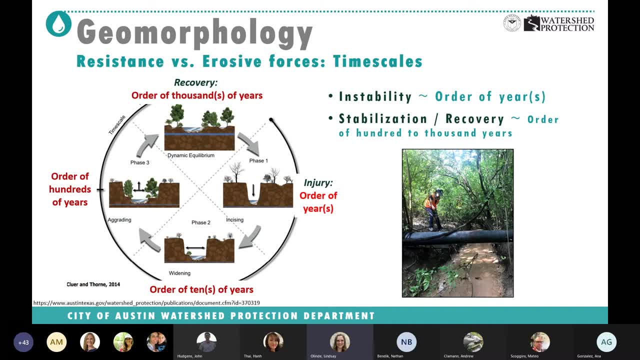 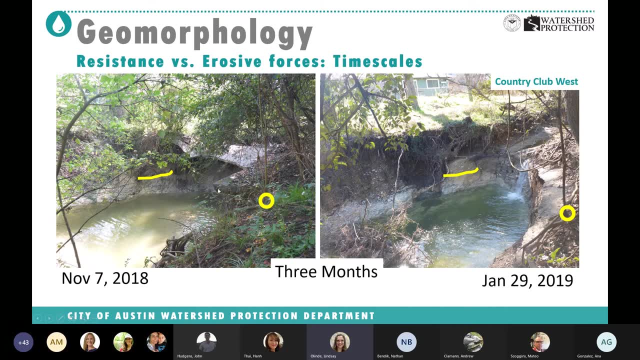 repeat what it did. We're going to let it recover And you know- and we've had a lot of volte and our first time with Ingrid- our next step is to catalyze that, either changing the hydrology or often kind of stabilizing and helping that recovery. This is another example where just 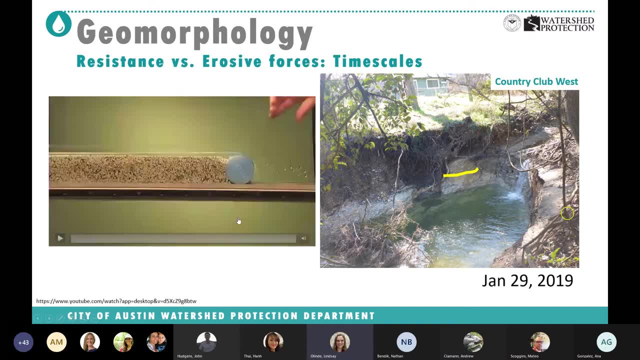 in a few months, just to show how fast this can change. This is an a few months. We were watching this head cut go through this old grade control in Country Club West And this is a great video. I feel like that just shows what's happening when we have these. 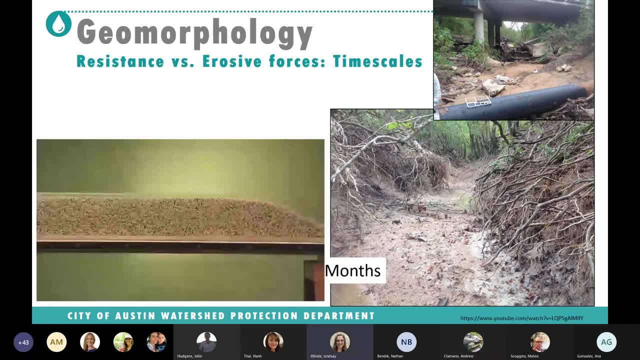 instability going upstream. This is another issue where, even when we had a forest in Gilliland, there was a head cut that started downstream and within just a few months the tree roots weren't strong enough to resist that head cut migrating through. The only thing that's stopping that head cut right now is this: 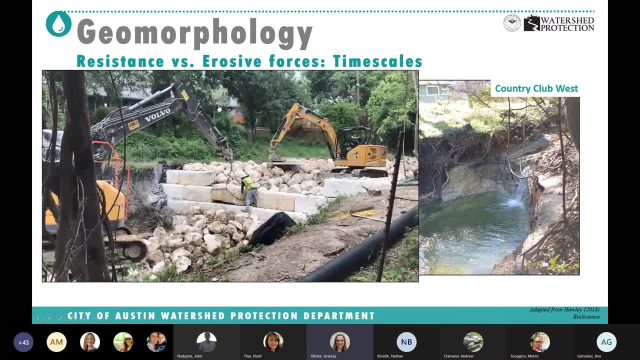 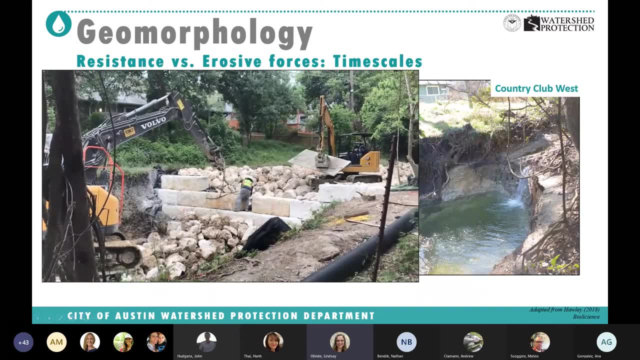 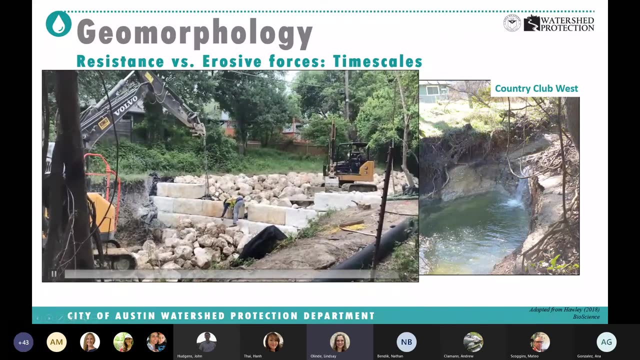 road is providing a grade control. Here's an example out in Catalina where we put in a grade control to try to stop that head cut that was starting to go through. and, as you know, this is really impressive and we're able to engineer this, but we can't do this at every head cut, so it's important that we can try to. 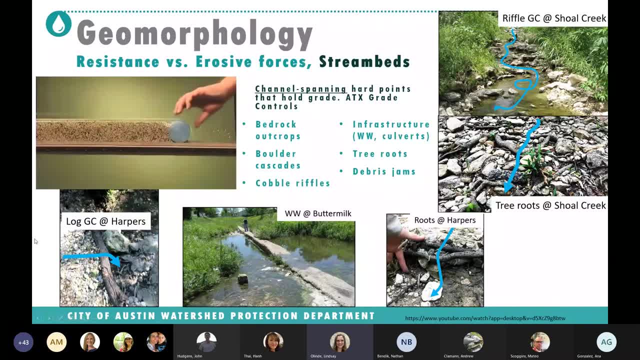 think about what serves as head cuts around Austin. We've got our bedrock outcrops. out west We have sometimes log jams. Every time I go to a creek and I see a grade control that is working, I feel like I'm in a great place. 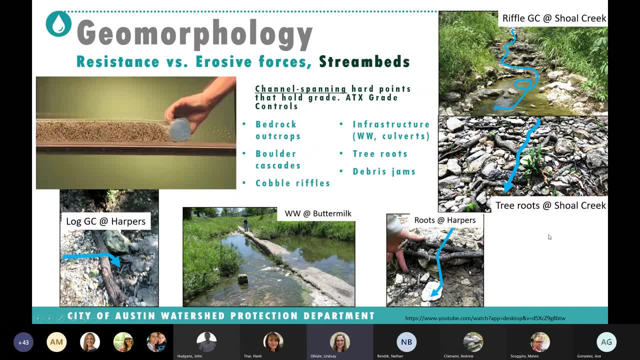 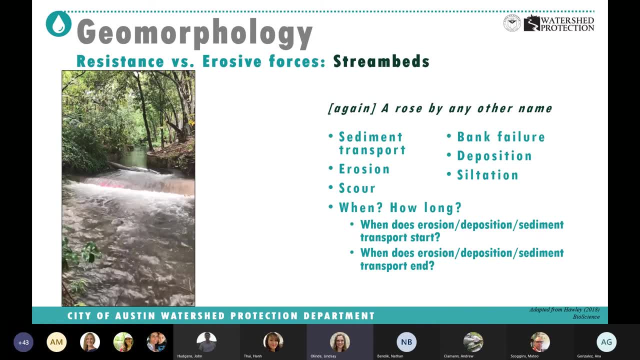 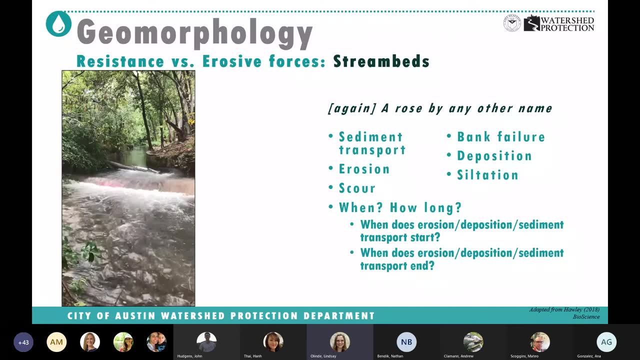 I feel really grateful. It can sometimes be as small as cobble riffles, depending on the stream dynamics. Stream beds erode and sometimes we can call it erosion scour. when it's a bank failure. eventually it's deposited. We want to know how long is it eroding, how geomorphology is really impacted by how. 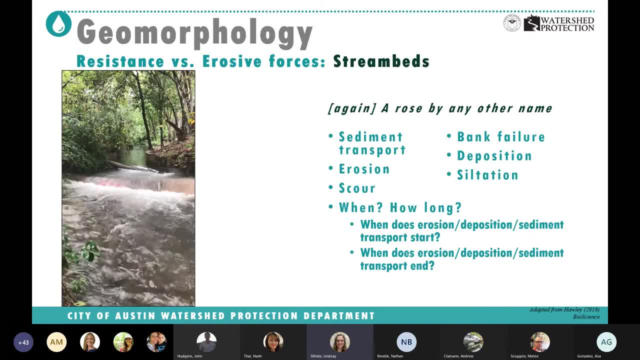 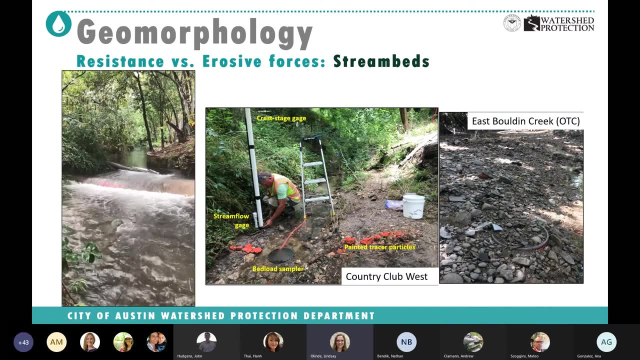 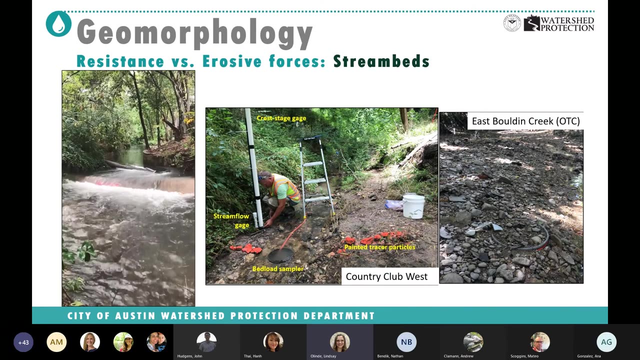 long erosion is happening, how much erosion is happening, how often erosion is happening. We have here's a picture of We're trying to- you know we have a project right now doing erosion monitoring- to kind of target and dial in how different erosion, that initiation of erosion and how frequent that happens across town. 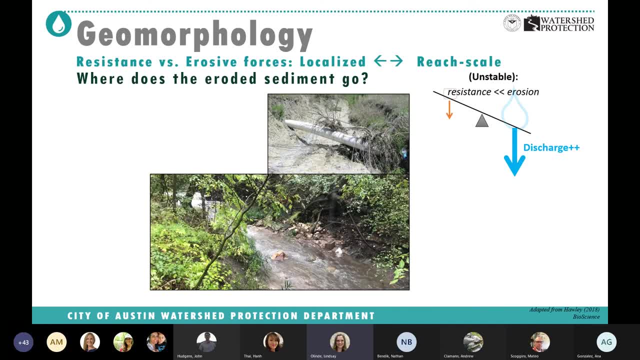 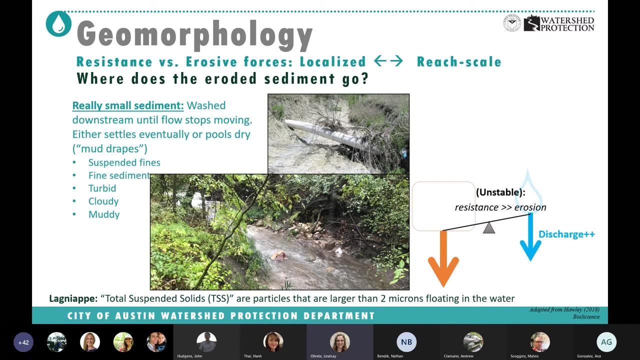 So we're looking at that now, And, even though I'm very erosion focused, it is important to remember that the sediment that is eroded doesn't just disappear right. It still exists, And so where does the sediment go? The really small sediment is suspended to fines. 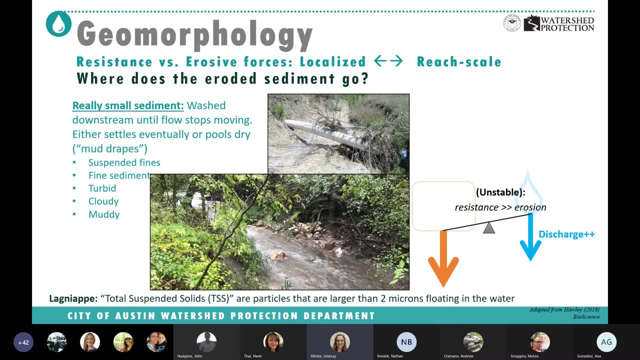 When you're in a creek, you might notice that it's turbid or cloudy. It's what's suspended in the water And that'll keep going downstream until the water is slow enough to let it settle out. And then we have coarser sediment, which includes sands, pebbles, cobbles. You'll see those in kind of like gravel deposits. 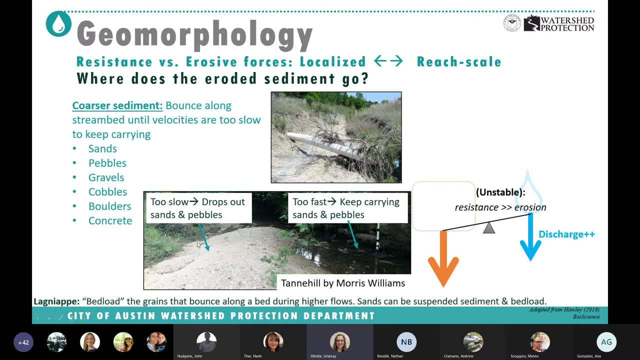 This is a great example of reading the creek, where, if you go out, you can see that In this space the flow was too slow And so it dropped out the sands and pebbles, But here it was too fast, So it kept carrying the sands and pebbles. 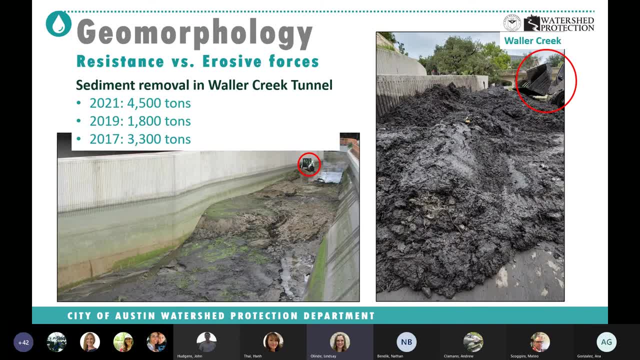 So all you have right there are the coarser sediment, Most obvious place of where we're getting. you know where does the sediment go? This is Waller Tunnel. We get, we have, tons of sediment that we have to remove And we don't know where all of this sediment is even coming from in Waller. 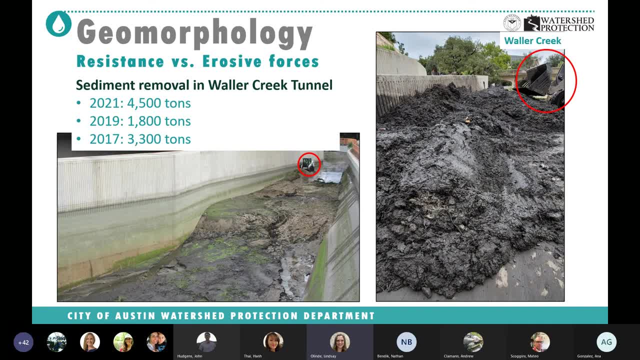 But we are managing it and having to clean it out. So this is a reminder that even if we have an erosion at some place, it has to. the sediment is going somewhere, And so that's important for us to remember. We have some streams that are looking pretty good. 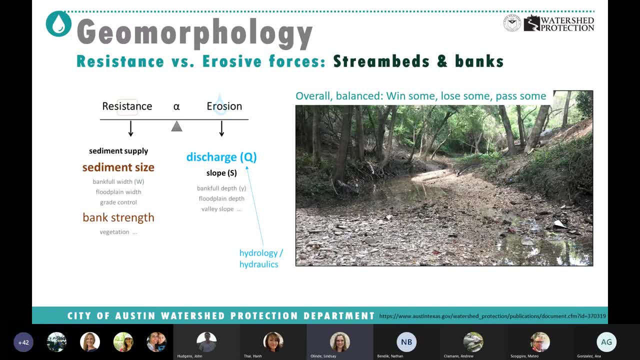 We've got kind of an overall balance where we win some, we lose some, we pass some. I'm talking about sediment here. This is one spot behind OTC that in general we have some access to the floodplain So you can kind of see, depending on what event, the creek is moving around a little bit. 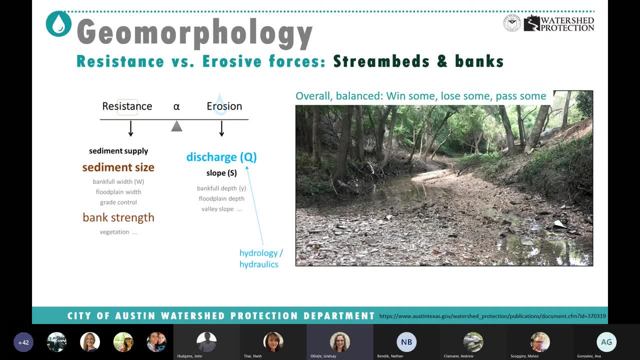 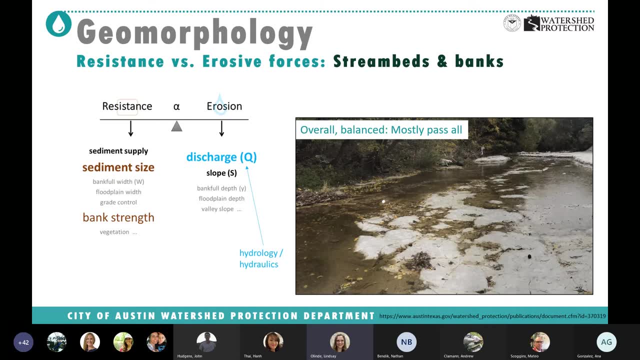 Not a ton of erosion, Not a ton of deposit, And overall it's pretty balanced. I would argue that even this is pretty balanced. This is a bedrock creek And we're just passing all of it through because it's so smooth. 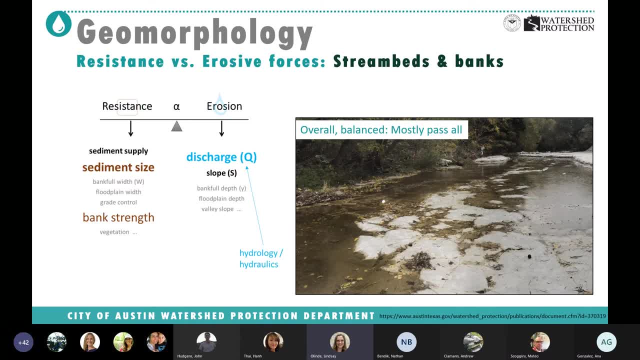 We have a lot of hydrology, But it's not super unstable in this particular section. Is it good for our ecology? No, Did it used to have sediment here? Yes, But right now it's still. it's out of balance in terms of just sediment transport. 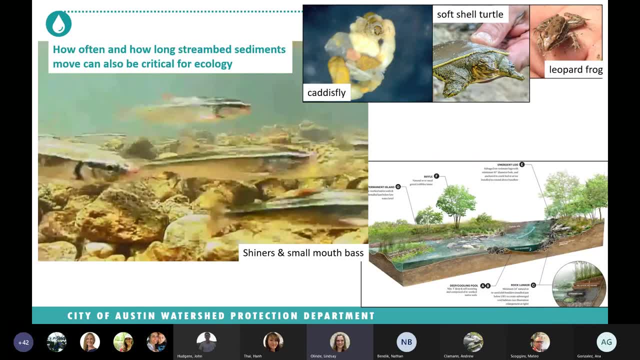 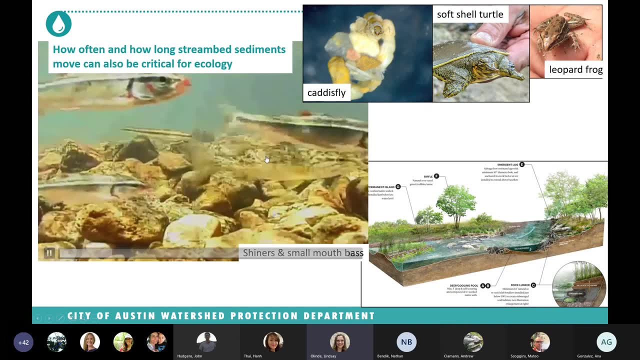 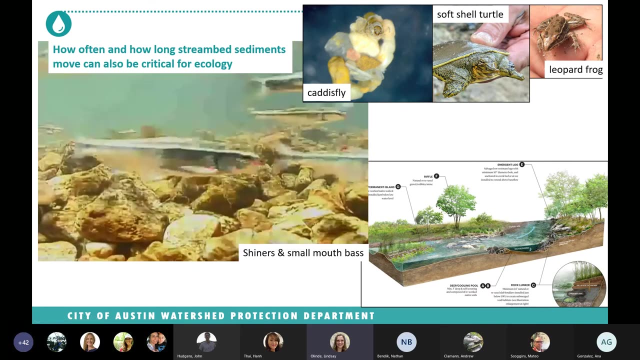 And that it's passing it all through, And this is an image that I love from the Missouri Department of Natural Resources showing gravel. I've got these little shiners, some smallmouth bass. I'm showing this because how often sediment moves is critical for a lot of our stream ecology. 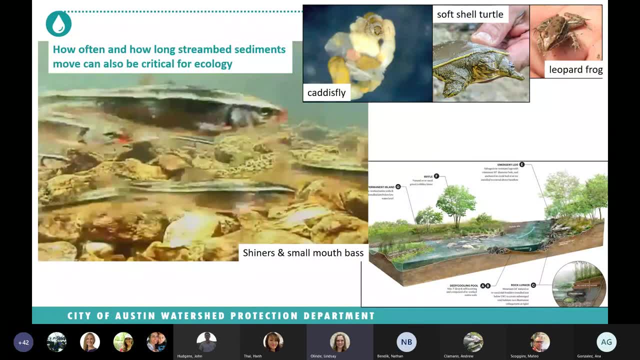 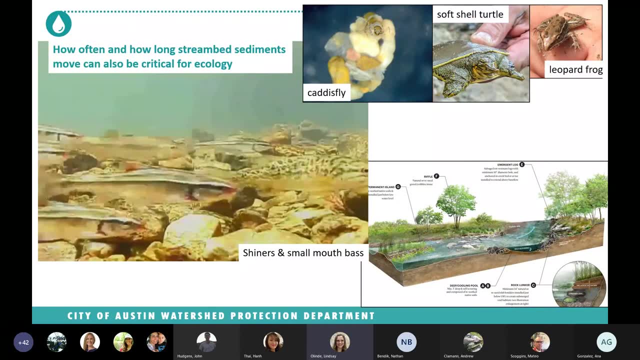 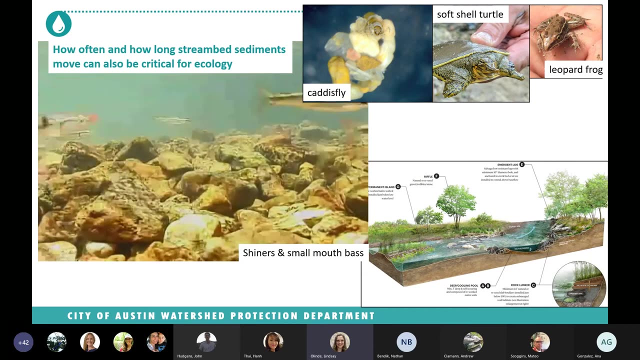 So how often those gravels are picked up and mobilized? that's just saying how often is it eroding, right? So when we have these small events that are super connected and then we're having these outfalls coming into our streams and we're getting these really big pulses, even with small events, that's different on an ecological timeline than what our macro invertebrates have been involved to withstand. 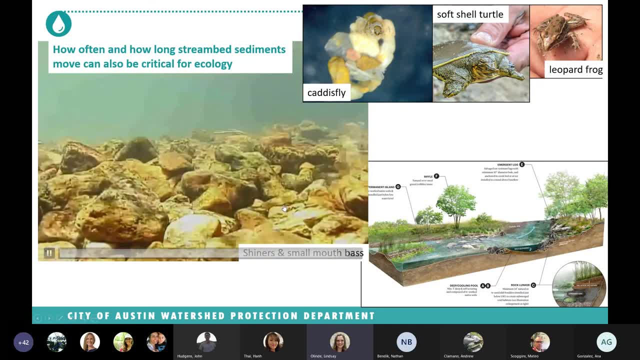 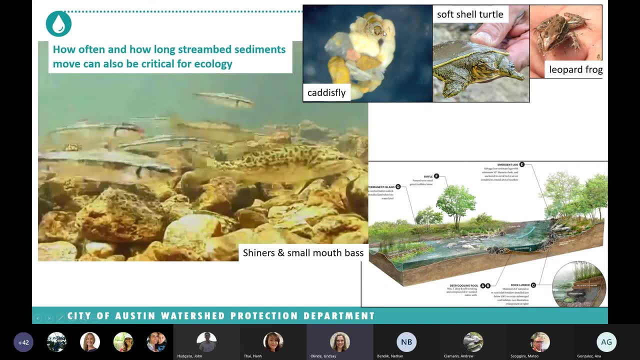 So if we're moving these gravels quickly, then that's changing how our ecosystem functions. Here's a great picture of a caddis fly And I'm going to show you a picture of a caddis fly. And this is a picture of a caddis fly. 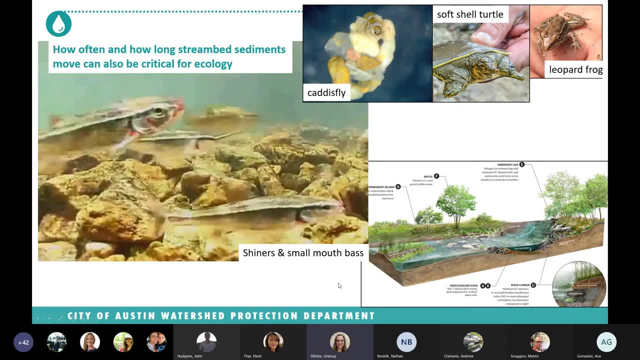 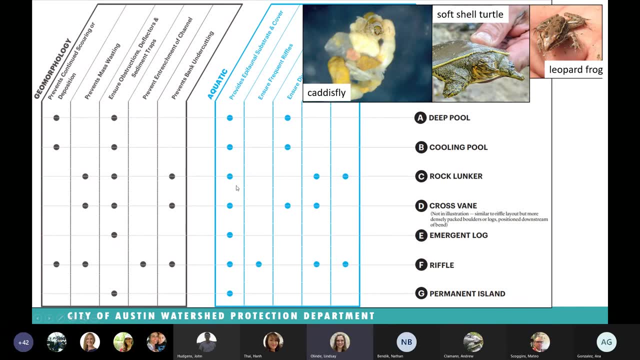 So thinking about that and I know that we'll link that and talk about that more as we go up the functional pyramid. This is also from my Waterloo Waller Creek love. They took those different components of the stream feature and they were able to connect it to both geomorphology- so kind of resistance. 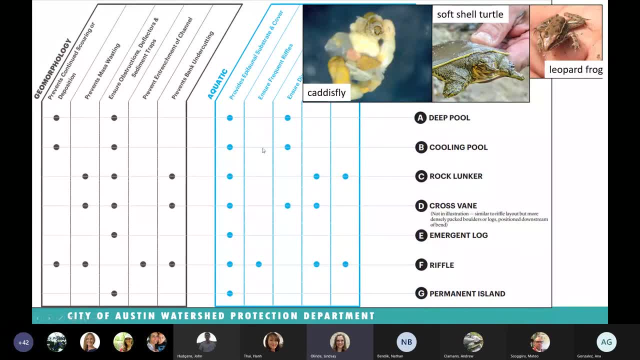 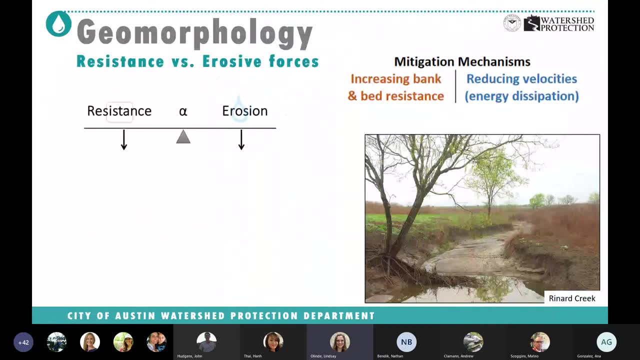 And then also our aquaculture, And I just really like how clearly that was connected. I often think about erosive and resistance forces when I'm thinking about how are we mitigating something, So trying to go through- probably a linear thinker- to a fault. 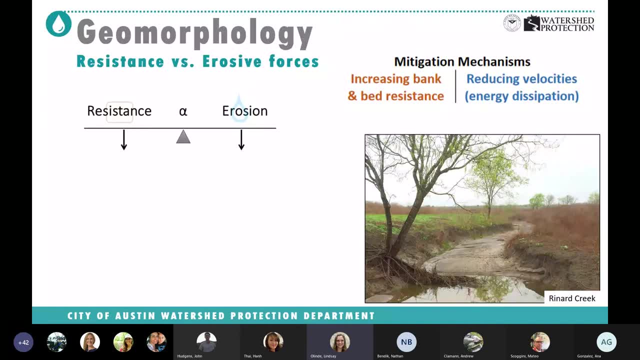 So I have to really break it down into processes Like: are we increasing resistance? Are we reducing velocities? Are we doing both? What can we do where? This is an image out of in Blackland Prairie, where we've had, you know, almost 100.. 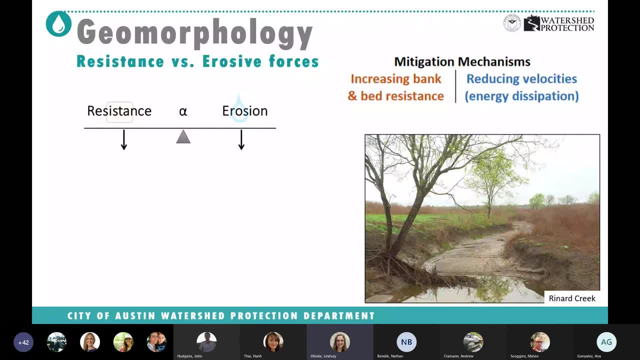 50 years of riparian forest loss. We don't have that bank stabilization anymore, We don't have that stream bed resistance that we would get from tree roots And we also don't have as much watershed kind of the watershed upland capturing the flow. 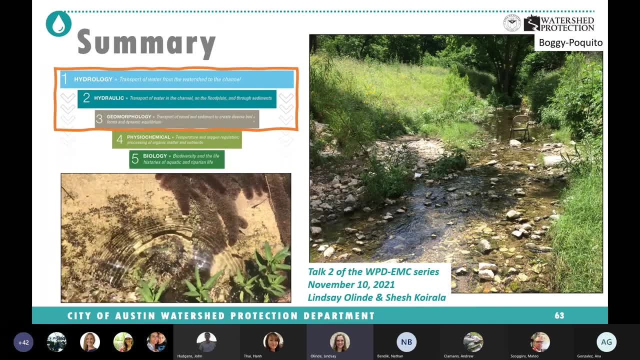 So we're having a lot of problems out there. Thank you for joining us on a stream, talk and walk. I hope you all learned something and I open it up for questions and would especially like to hear Hear from folks who maybe don't think about geomorphology as often. 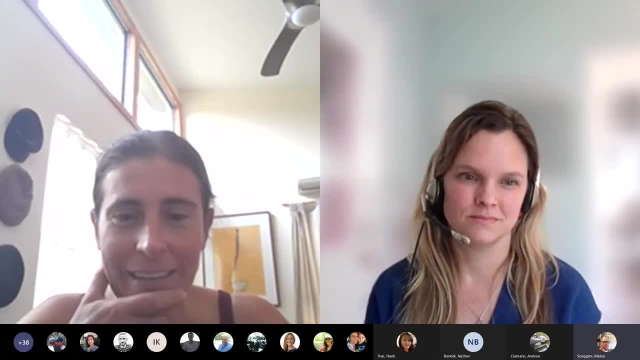 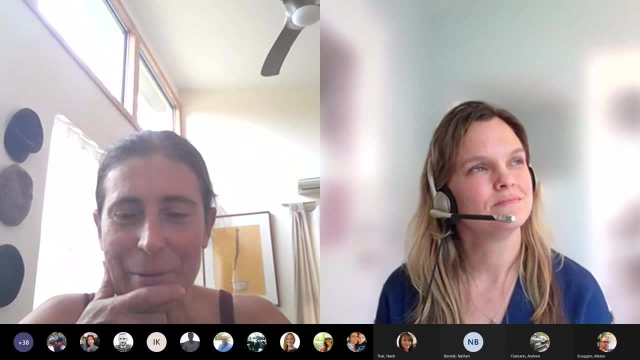 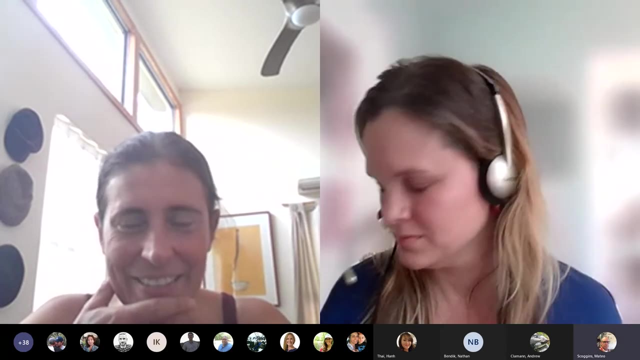 Todd made a comment yesterday about caddisflies and resistance. Do you remember what his comment was? Maybe Mateo can remember, since he knows more about caddisflies than I do. Do you remember? Is it like stream bed resistance? Well, yeah, 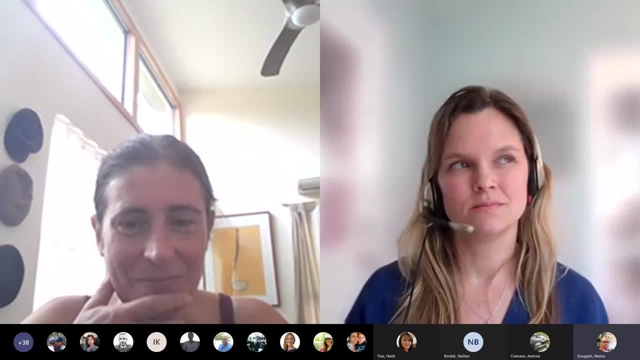 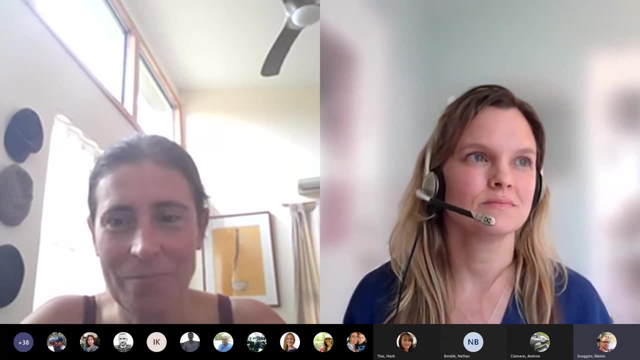 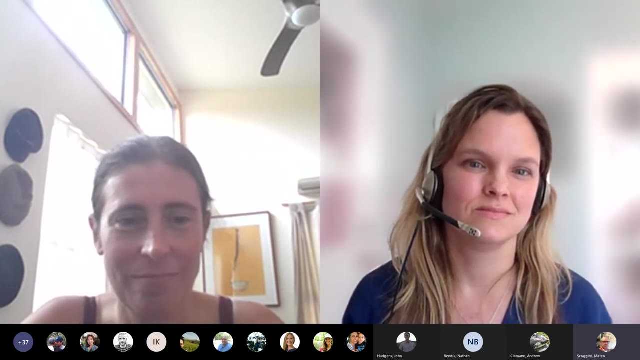 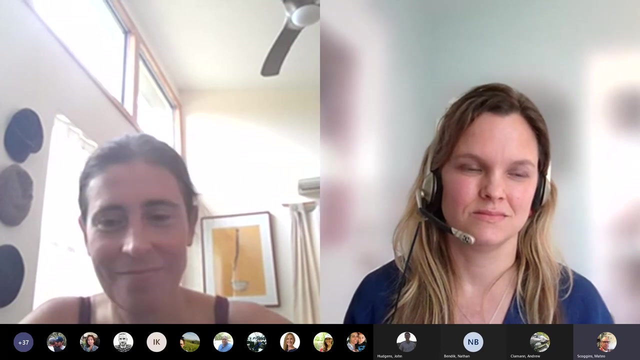 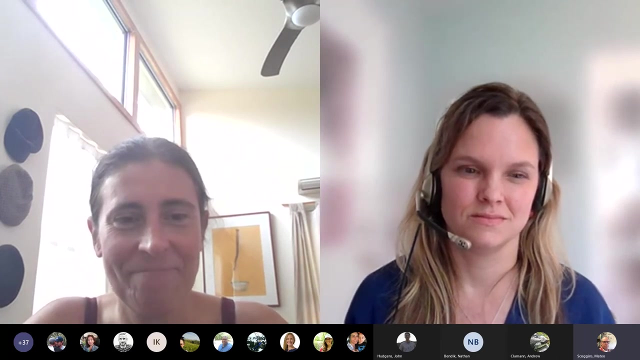 The comment was how ecology can play even a more kind of physically functional role in stream. Yeah, So we've been seeing a lot more of these kind of extreme systems than people really realize. A lot of the net spinning caddisflies- we have a few here in Austin. they actually can get so dense and make such an array of nets that they can move that kind of boundary layer of velocities up above the substrate and actually change the way water flows through these streams. 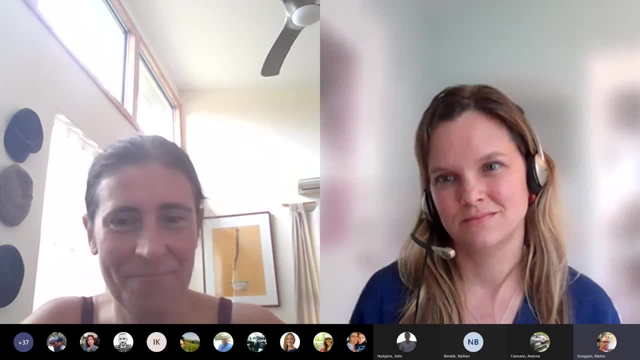 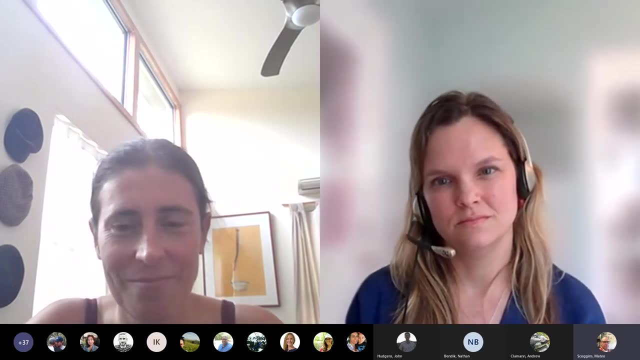 You know it's on a smaller scale than maybe Beaver or some of the other engineers that we have, but they definitely affect the stability of some of the kind of substrates and riffles systems that we have in certain streams. yeah, for like those, those west. 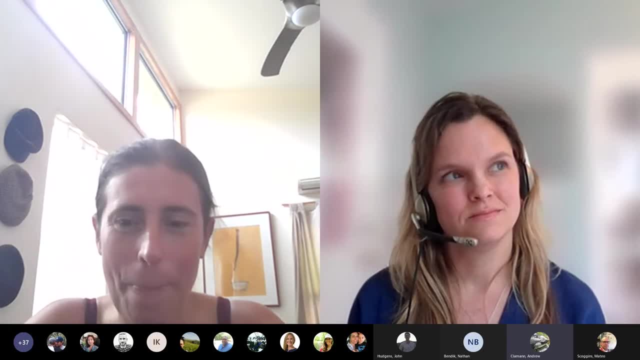 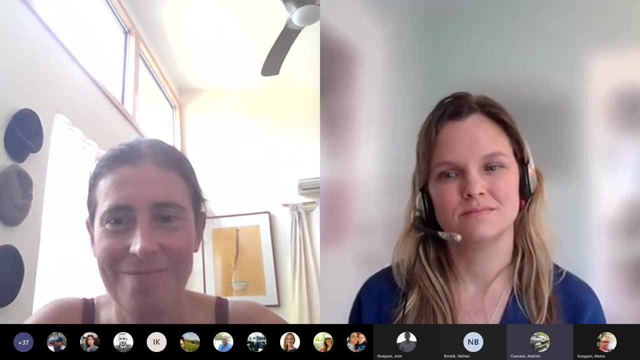 side streams that are really flat and really wide and maybe only be a half an inch deep, maybe an inch deep, but you're still pushing through. maybe you know five or six cubic feet per second just because the stream is so wide. but when you have a bunch of these little, they look like little tents and they're all. 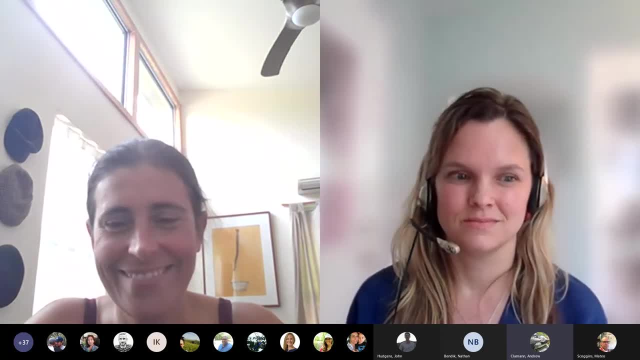 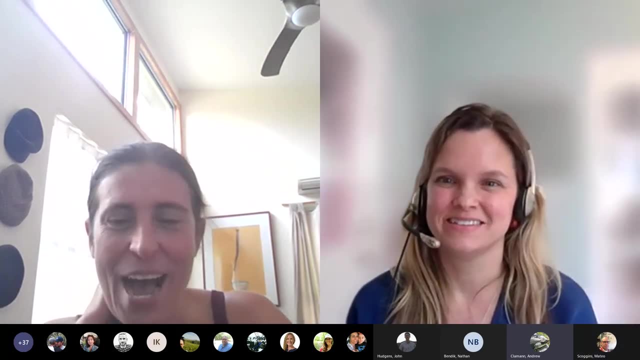 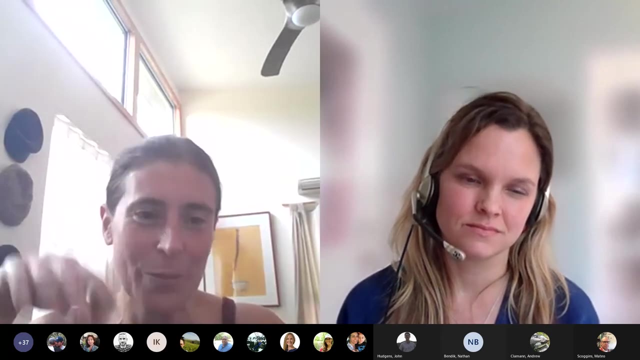 facing upstream and they all catch water and so they cause water. then stop and bump and go over them. so, um, tiny, itty bitty beavers- yeah, thank you. i actually have a question, uh, on that. those ideas of you know how biology feed, but it fits back into providing resistance. you mentioned that, um, in in that blackland. 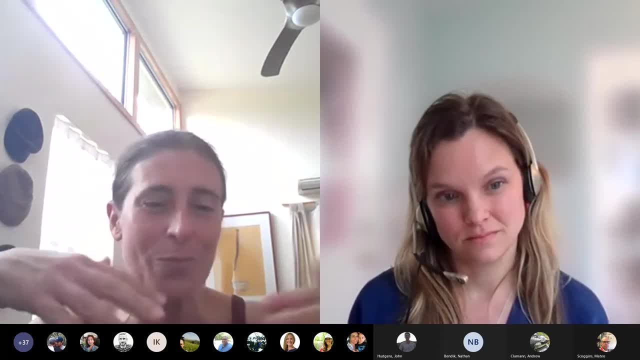 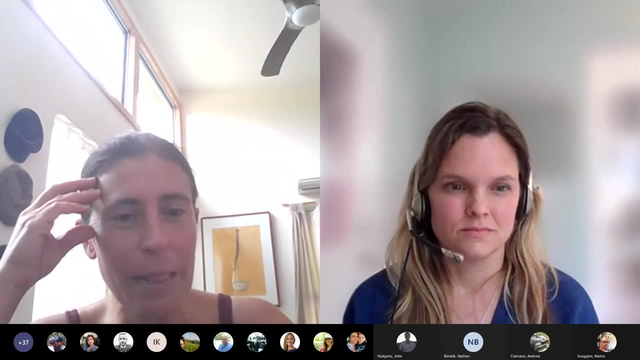 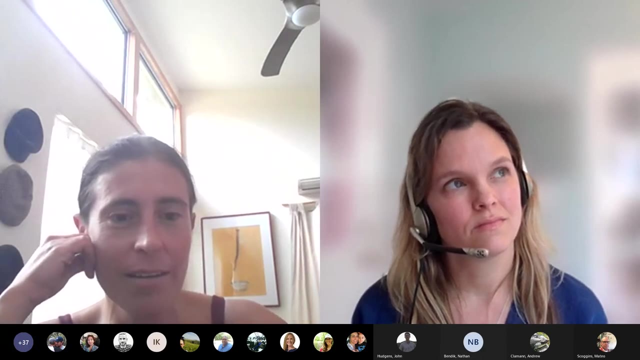 prairie creek, where the trees were no longer able to sufficiently provide that resistance. can you speak a little bit more on on the role that uh biological elements such as trees uh are an important component, depending on what ecoregion we have in our in our area? i was really surprised, um, i've been working on blackland prairie. 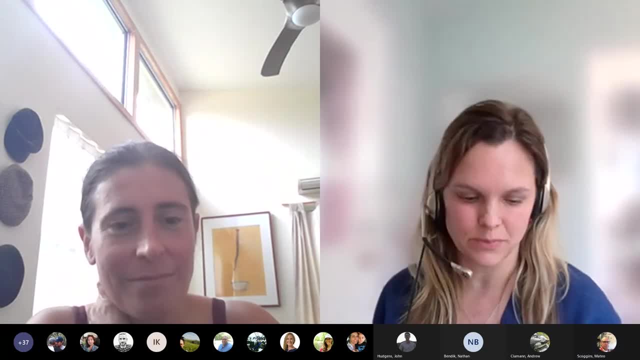 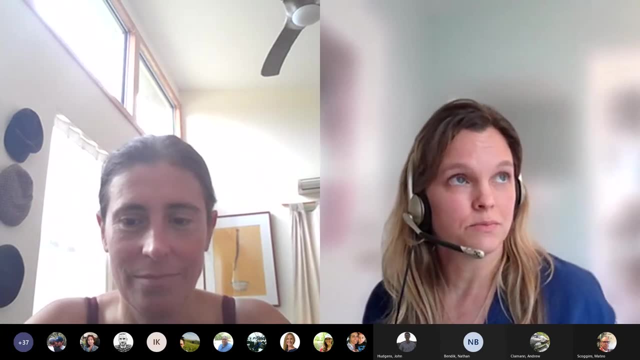 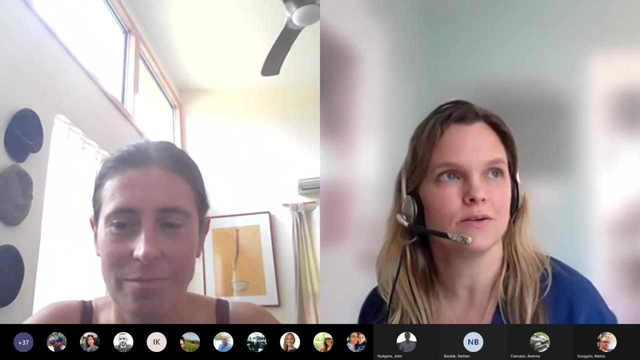 geomorphology and vegetation over the past couple years, recently put out a report about it, but to be honest, i have always thought of stream banks being affected by trees, um, and having that strength you can imagine like cypress roots along the edge or you know any kind of stream roots, but i think it's 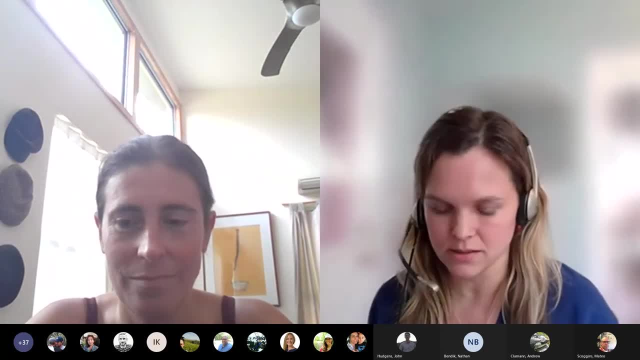 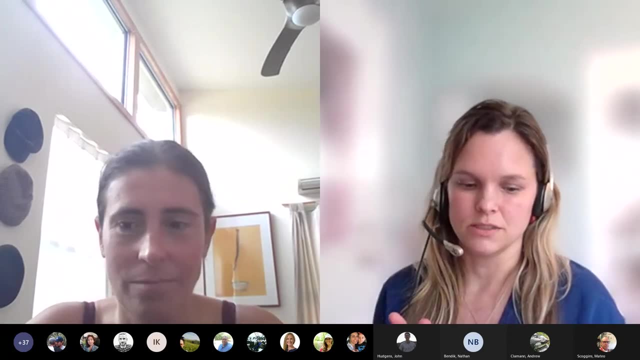 that's a pretty big difference. but i found that in blackland prairie- and i've started seeing this kind of across austin, even in um the west- we have a lot on the narrower, the narrower streams. we have stream roots going through and in the blackland prairie 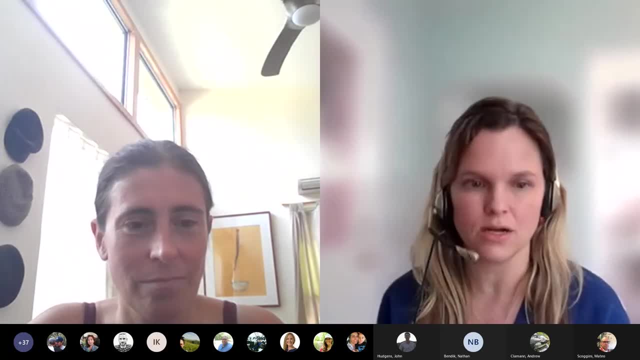 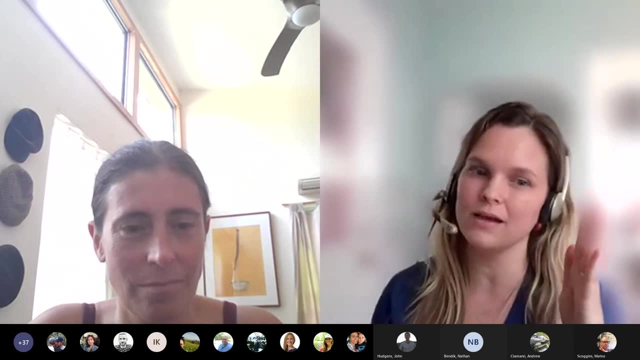 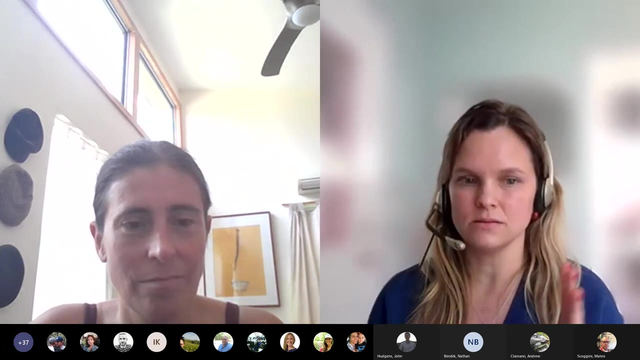 we don't have a lot of. we don't have bedrock outcrops, because we're in a different ecoregion. all that limestone that we see out west is there, but it's way down. so we have these, this huge hens of alluvial and um kind of clay that we can start cutting into the stream. so, naturally, the 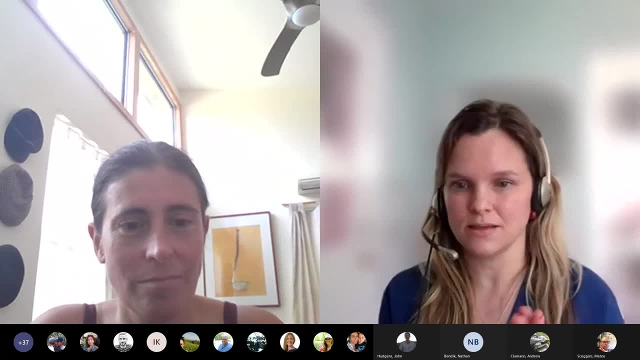 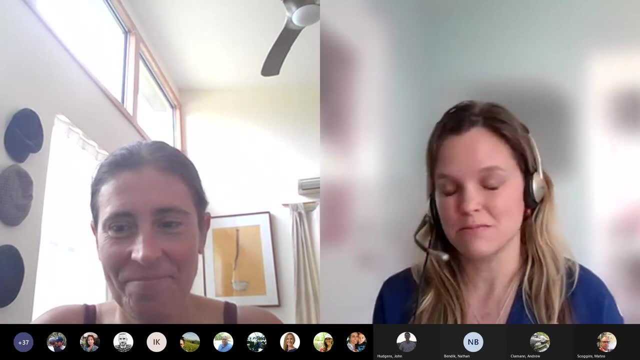 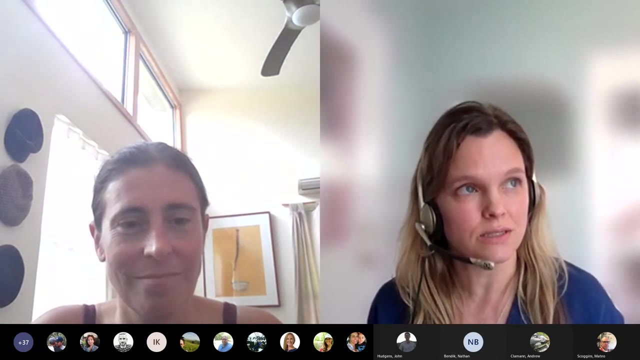 only hard point, hard points that used to exist in the blackland prairie were our riparian forests, which- spoiler alert- um, i have been able to find a ton of historic writings on what did the blackland prairie creeks look like and the and the most of them are from like the early settlers and 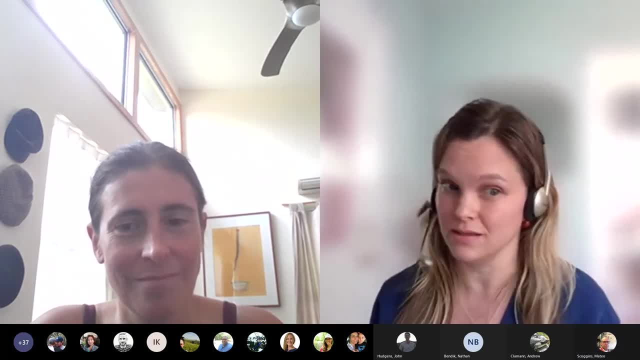 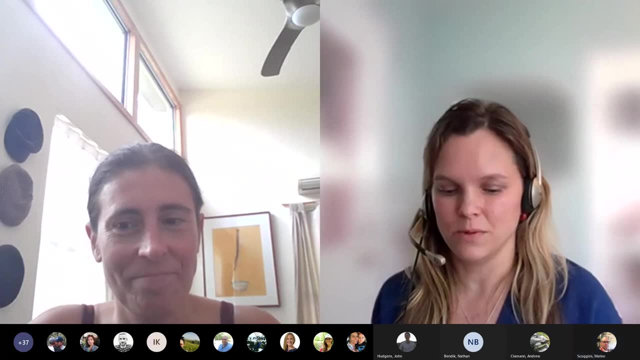 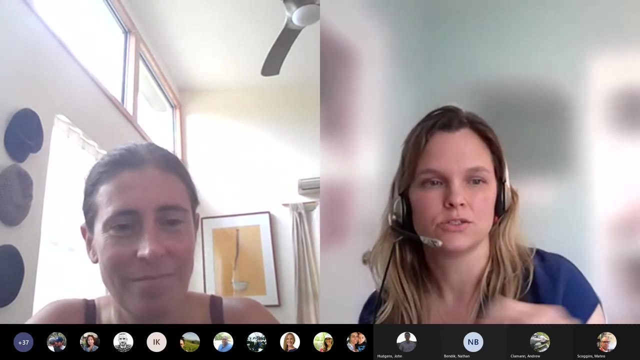 they all describe something different than what i am used to thinking, which i used to think: oh, prairie doesn't involve trees, um, but we have a ton of records where the blackland prairie was covered in these ribbons of trees and riparian forests, and we have early settlers even describing water flowing through there as clear, which is just like to me. it was a total shift, um. and then i thought about the processes. it really makes sense. prairies used to be, um, you know, really the grassland part would be a soaking in. so you're taking that um kind of erosive force piece of it. 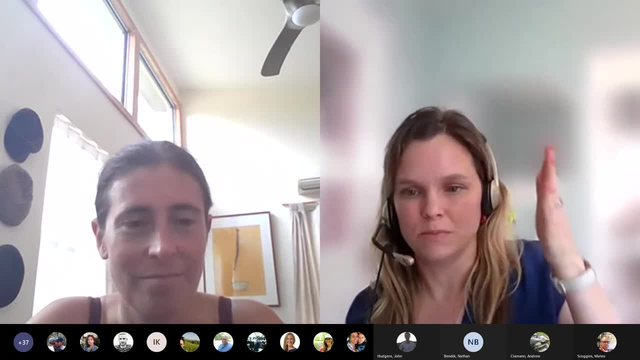 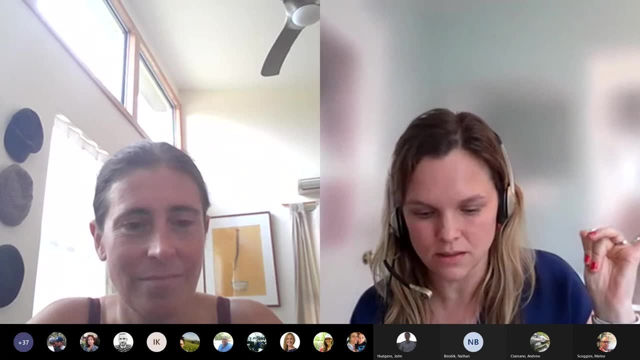 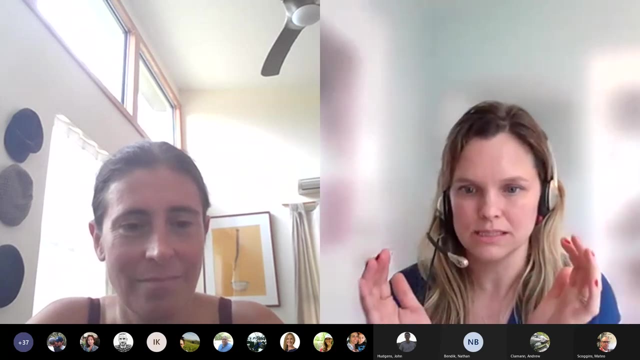 and then the riparian forest that used to be there would have been both resistant on the bank and resistant across. so, even though the particles are much finer than what we would see in west austin, we had that balance both on the watershed scale and on the resistance. 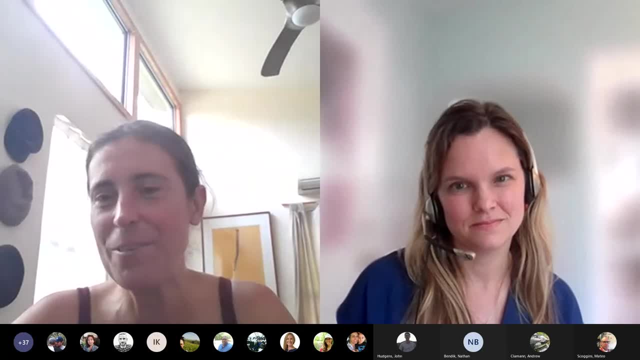 of um the blackland prairie. thank you everybody for for attending and stay tuned. there will be more presentations coming in.